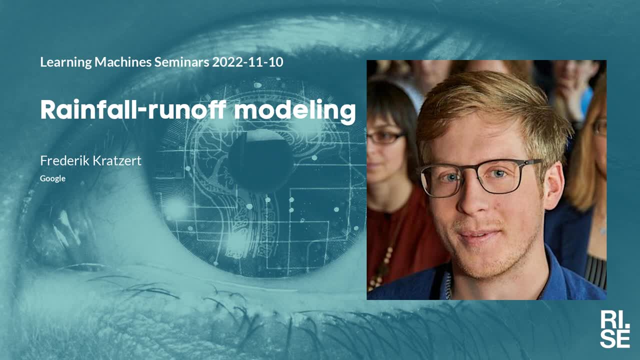 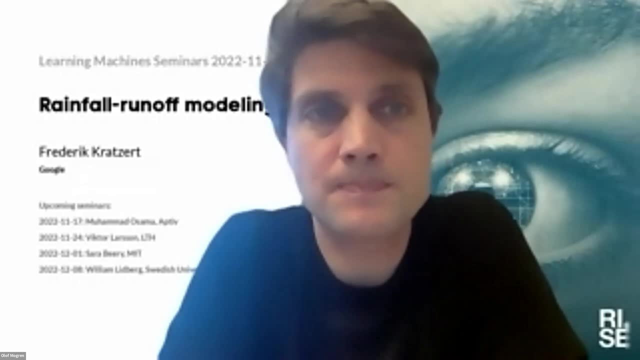 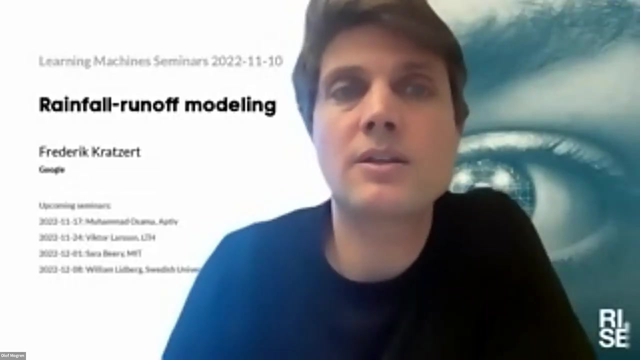 Welcome to RISE Learning Machine Seminars. RISE is Sweden's research institute with 3,000 people working on topics spanning from bioeconomy to digital systems. Specifically, the computer science department works on applied AI projects for the benefit of society, and we organize the 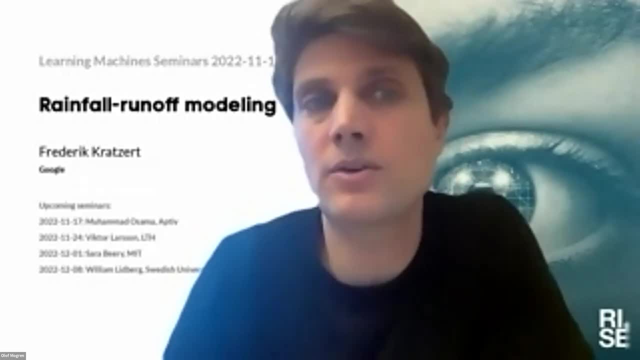 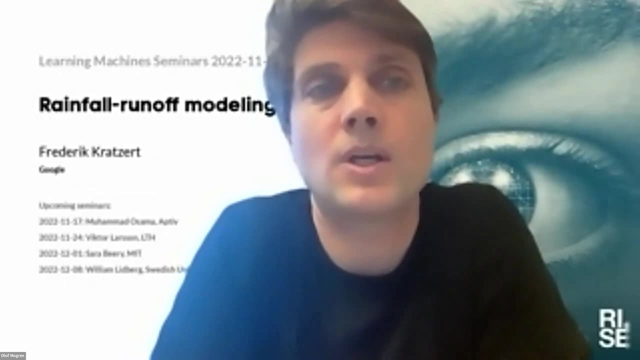 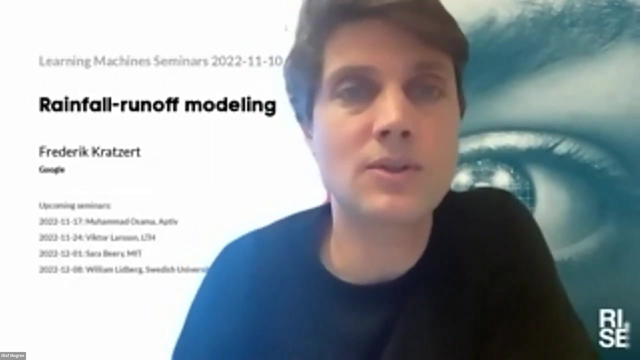 weekly Learning Machine Seminars as part of our Center for Applied AI Research. This meeting will be recorded and if anyone wants to be removed from this recording, please let us know. Otherwise we'll put it on our YouTube channel, which you can check out to see a lot of nice talk. 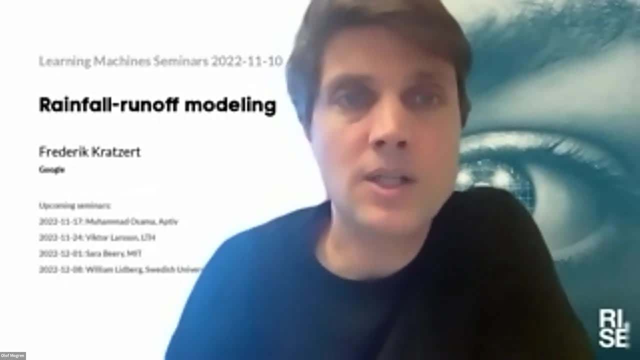 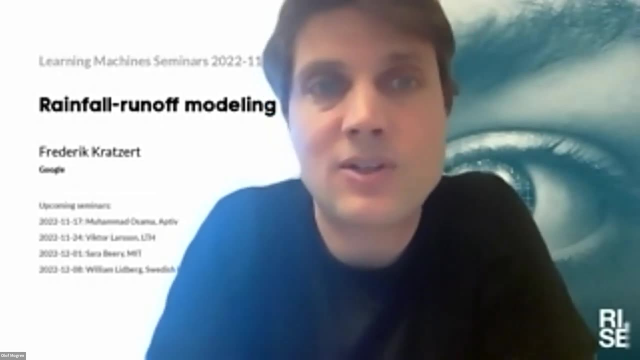 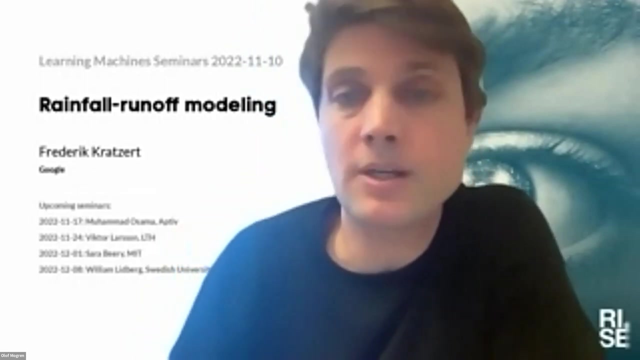 which we've had in this seminar series. Today, I have the pleasure to introduce Fredrik Kraxelt, who is a visiting faculty researcher at Google in Vienna. He defended his PhD in 2021 at the Johannes Kepler Universität, Linz under the supervision of Sepp Hochreiter. The topic was deep learning in 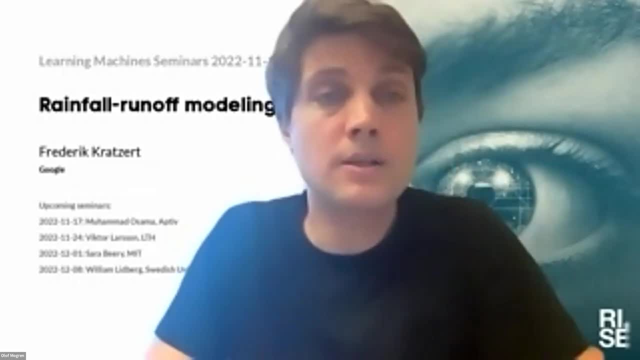 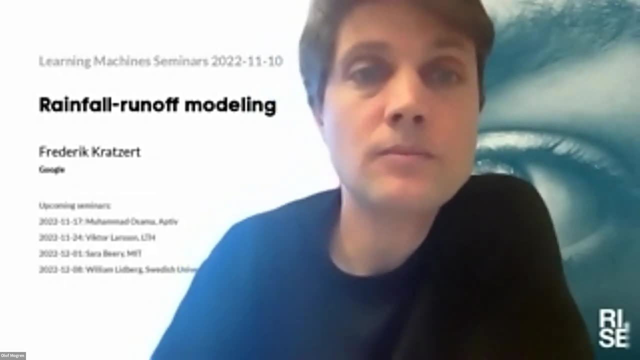 hydrology. He's currently working on the flood forecasting team at Google, who is building a global flood warning system, And the topic today is long short term memory networks for rainfall runoff modeling. With this said, I will hand over the word to you, Fredrik. 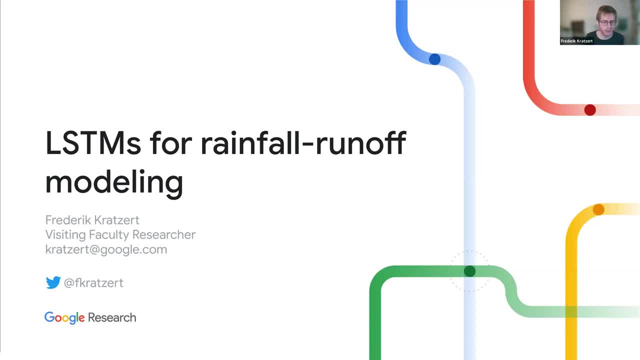 Thanks for the introduction. I welcome everyone on my side. Yeah, as Olaf said, this will be about LSTM-frame runoff modeling. It will be more talk from the application side of deep learning in this hydrologic specific decade And, as far as I understood, not everyone is a hydrologist or geoscientist in this audience. 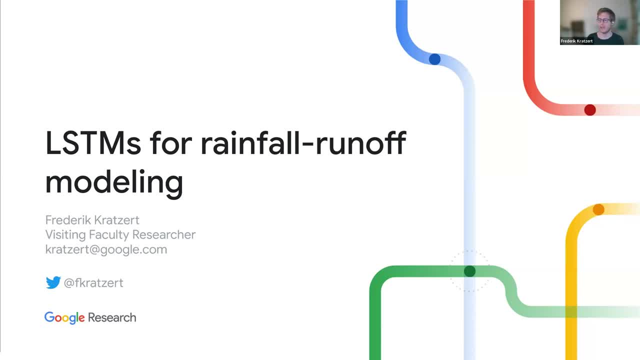 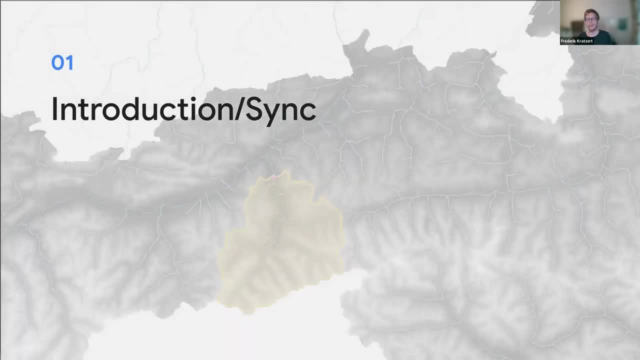 So I'm trying to get everybody on board with my introduction. So let's see, Yeah, the first thing I'll start with will be an introduction on describing the problem that we're trying to solve and what's meant for runoff modeling and why it's important. Also, feel free to interrupt me at any time. 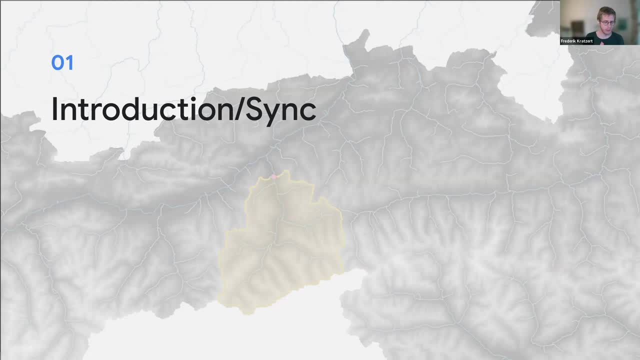 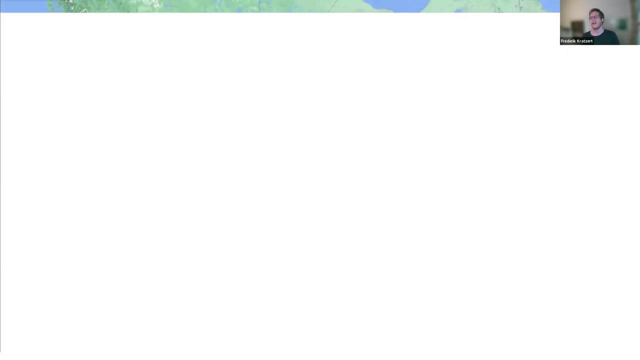 Thank you for asking me, 그 connector. I want to thank my colleagues for asking me specific questions. You can also write in the chat and then Olaf will read out the question and please excuse my voice. I'm like on the edge of getting sick and lost my voice today, So, yeah, it's a bit shaky. 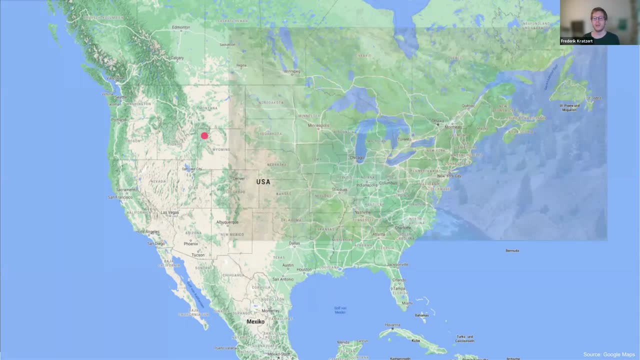 Okay, so what's rainfall runoff modeling? Imagine you're looking at the map and you point to any random river And now you want to know how much water there is in the river Today, or how much water the sea has today or tomorrow, or how this river has evolved in the history or will evolve in the future. 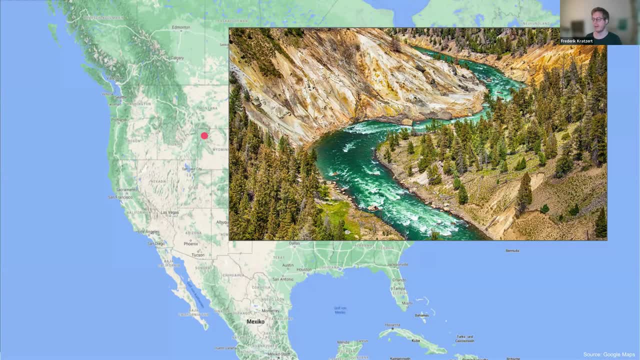 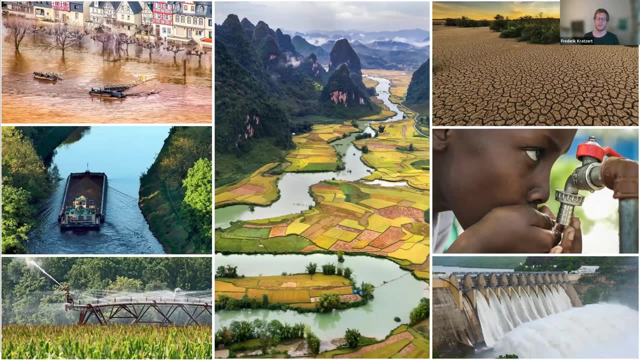 So this part of science is exactly what rainfall runoff modeling is trying to answer And, as you can imagine, rainfall runoff modeling is important for a couple of reasons: for society, and there are some more obvious reasons which are, for example, flood forecastings, drought monitoring and drought forecasting, But there's also water resource management for agriculture or 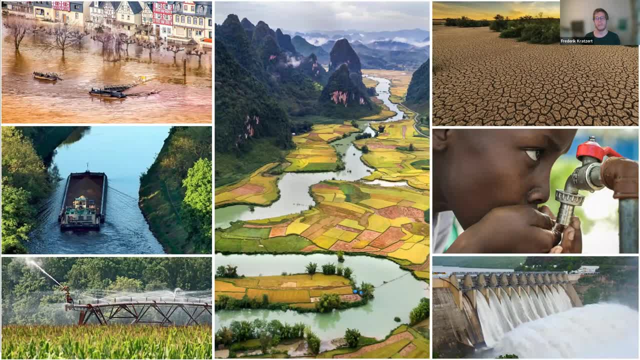 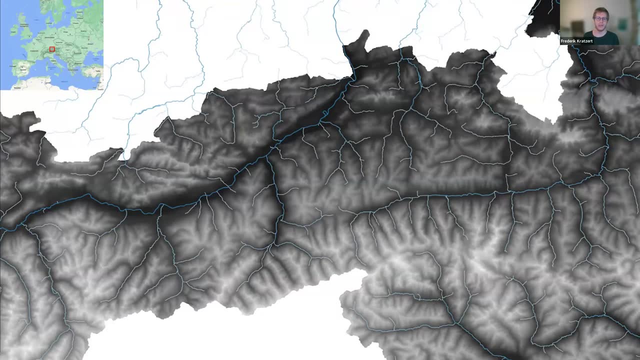 hydropower And, as I mentioned previously, some probably not so obvious reasons, is also that rainfall runoff modeling is used to estimate the future behavior of rivers under climate change. So for the rest of my talk, there are a couple of concepts that are important to understand. 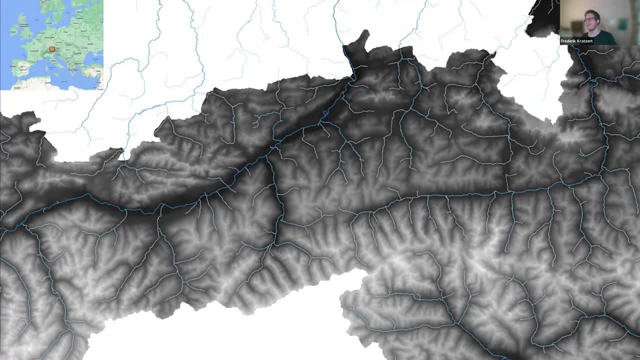 and that I try to introduce on this slide. So what you're seeing here is that we have a digital elevation map of parts of the Austrian Alps and light colors mean higher elevation and dark colors mean lower elevations. So let's imagine we are interested in the discharge at the 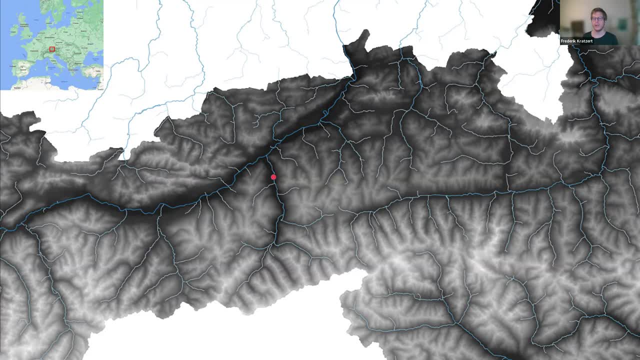 red point in the river. Now, this green color at this point is influenced by only a specific area, and this area is called a catchment or a basin. And for simplicity, let's say this area is only defined by topology, meaning that any point of precipitation that falls within the yellow area will at some point 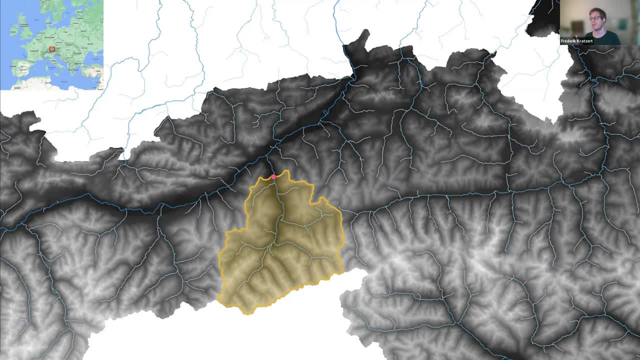 reach the red point in the river or will be lost here to evapotranspiration, but it will not go to a river in the neighboring valley right. So this yellow area is called a basin or a catchment, and in higher elevation this yellow area is called a catchment or a basin, And in higher elevation, 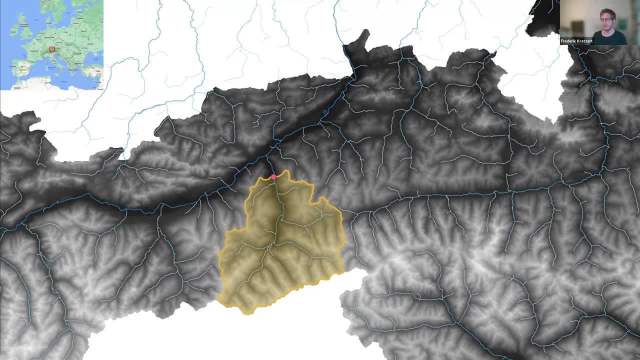 this yellow area is called a catchment or a basin, And in higher elevation, this yellow area is called a catchment or a basin, And, in higher elevation, probably the most common modeling setup if we want to model the river stream flow at the red point. 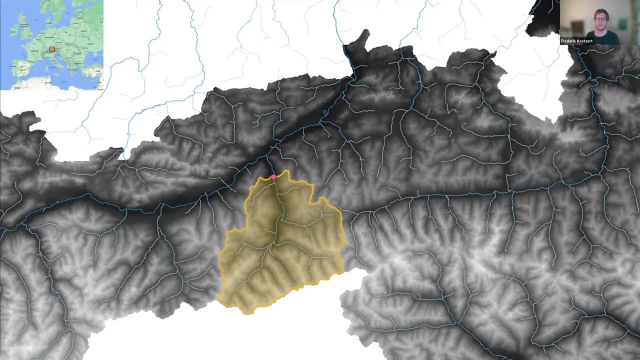 is to model this entire area, what we call, not meaning that we average all inputs across space in the yellow area and model this entire thing as one entity, So we lose the information about where the precipitation falls, but up to a certain size of catchment area this has proven to work quite well. 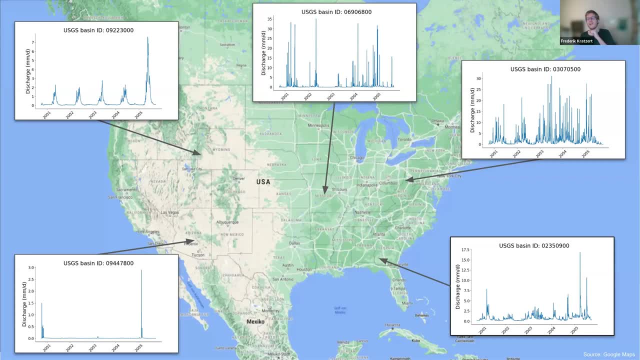 So if you can imagine, depending on where we are in the world and on the environment and the climate, So if you can imagine, depending on where we are in the world and on the environment and the climate, natural rivers behave quite differently. So you can see, in the lower left in Arizona we see the 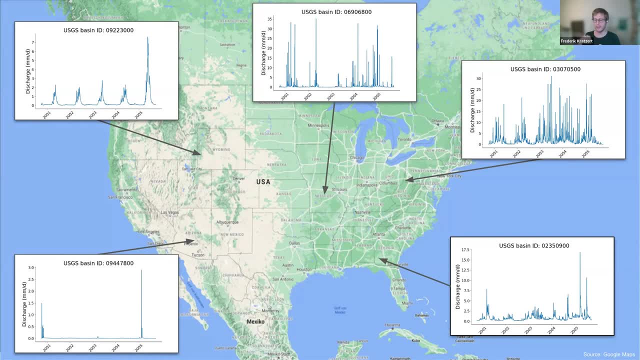 hydrograph. A hydrograph is the time series of discharge in a river. You see the hydrograph of an arid basin. So in arid basins we have extended periods of complete dry fall, of zero discharge, and then, with certain precipitation events, we have immediate spikes in the discharge signal. 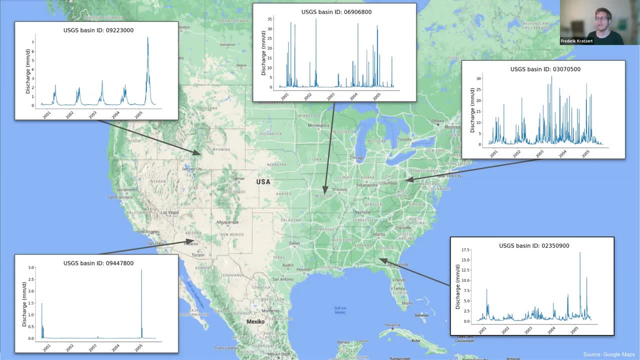 And then in the upper left we see a catchment of the Rocky Mountains, a very typical hydrograph of a seasonal snow-influenced catchment with very low flows during the winter period and then during spring and summer the snow melts and we get the summer peak discharges. 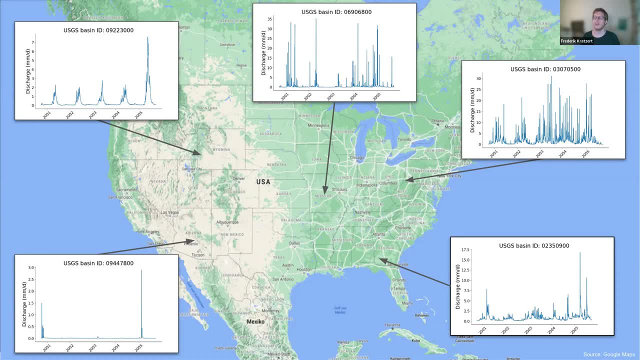 Now, if we want to model all of these hydrological systems, we need to incorporate a couple of different hydrological processes that influence the river in these areas, because in all of these areas different hydrological processes are important, And if we want to build a model that can model all of them, 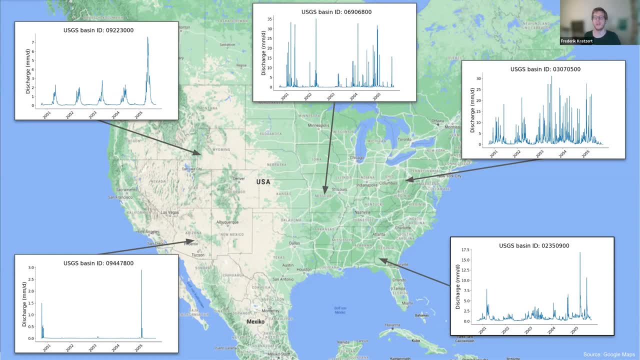 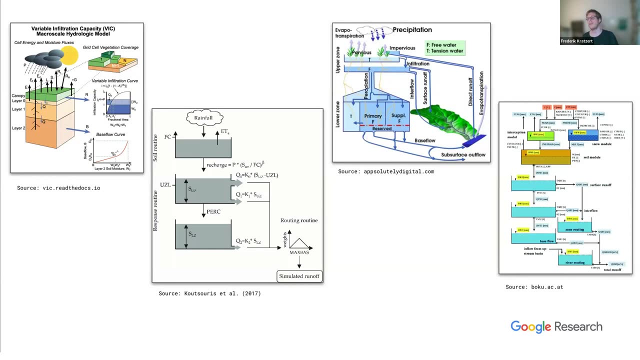 we need to know and implement all of these processes. At least this has been the case so far. So hydrologists, over the last couple of decades, developed a plethora of physics-inspired models, And the most common type of models is what we call bucket-type models. or, yeah, bucket-type models. 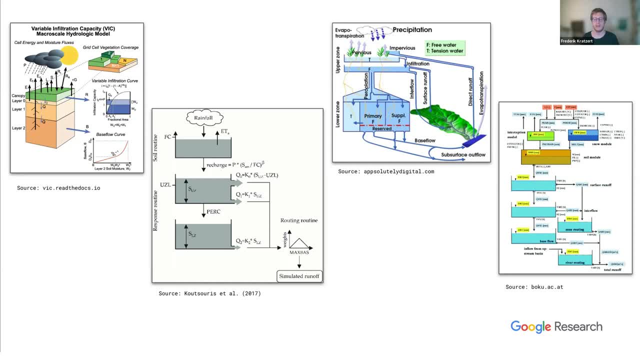 So here different states in the real worldate snow or soil moisture- are represented as buckets or storages in the system. There is also another common type of models. Pier contributes to the developing of these processes and then the transition functions between the inputs or in between the buckets. 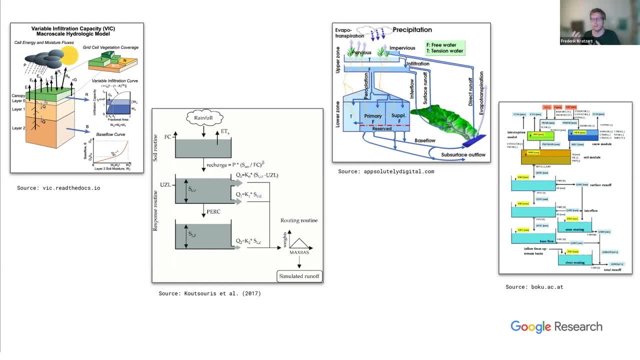 are predefined by the user, by the hydrologist, actually by the model developer, And the entire model only contains a handful of parameters. These parameters are then calibrated using some historical observations, and the inputs to these models are usually just precipitation and temperature. So these models 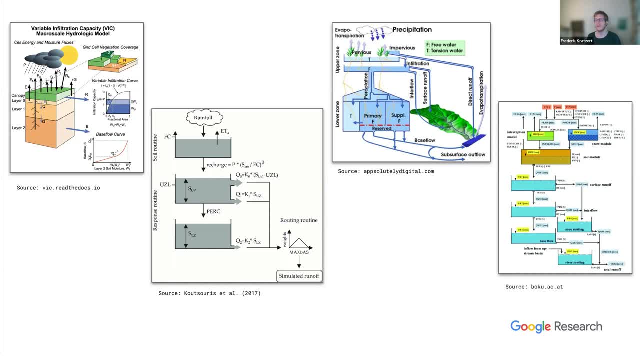 then have to model all the processes. The output of the model is the discharge. Yeah, so here I think there are no hydrologists. so I'm probably not making myself unpopular here, but I would say over the last two or three decades probably very little has happened. 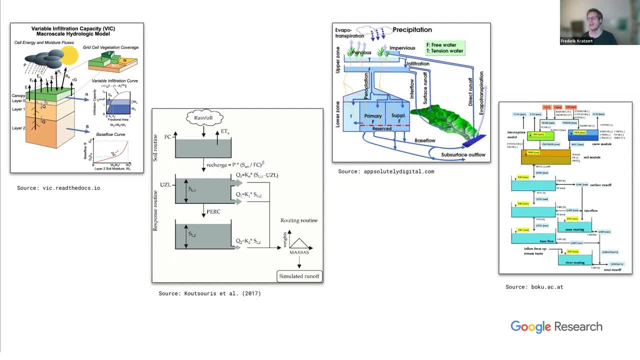 in the space of model development and hydrology, And the models that are applied operationally in hydrology are generally not as good as the models that are applied operationally in hydrology are still the models that were developed in the 70s or 80s of the last century. 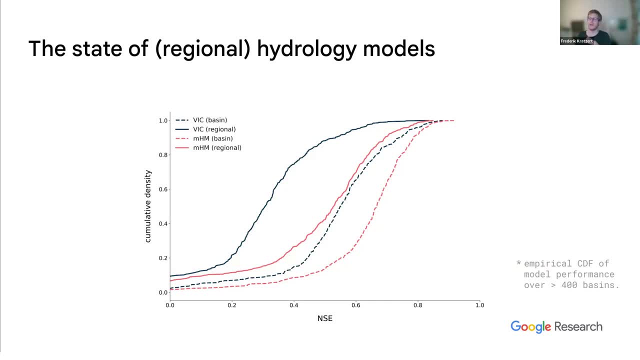 So let's have a quick look on the performance of hydrology models on a large sample dataset. So these kinds of plots- we will see a couple of them in my presentation, So I'll take a few seconds to explain them. So what we see here is the cumulative density function of some models over hundreds of catchments. 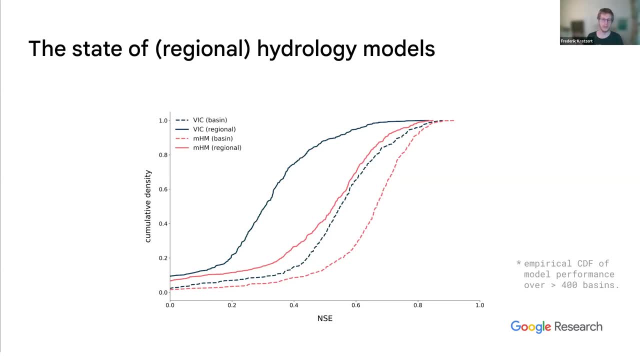 of the NSE metric. So on the x-axis you see the NSE, which is, for all non-hydrologists, just the air square. So hydrologists like to give it a different name, but it's just the air square. 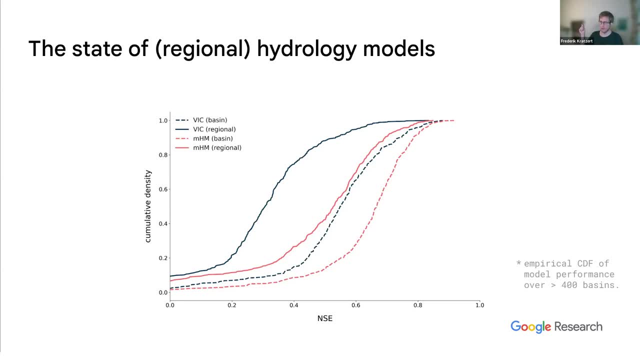 So NSE has an optimal value of 1.0. And a value of zero means that the model is stable. It's as good as predicting the mean, And everything below zero means that the model is worse than predicting just the mean. So what we see here is the CDF of two different models, and both of these models were calibrated. 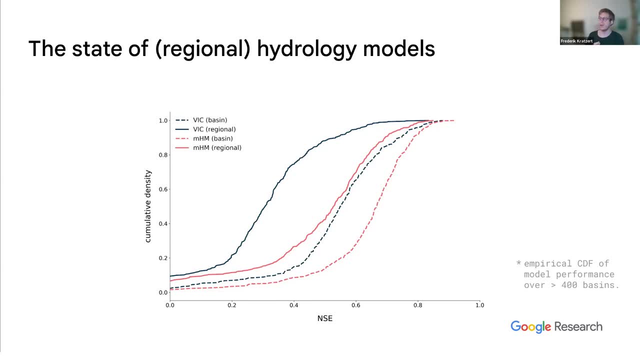 in two different ways. One is the dashed line. So here the hydrology model was calibrated for each of the basins in this dataset individually. So the model is calibrated, The model parameters were adjusted for every of these basins individually And the solid line is the same model, but the model being calibrated in a regional fashion. 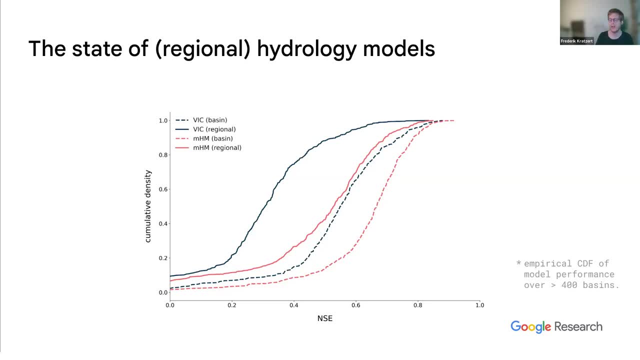 meaning that we have a second, what we can call a metamodel, And this model receives some auxiliary inputs, or it learns some transfer functions And then, given these auxiliary inputs, it outputs the parameters of the hydrology model. So it's basically one model. 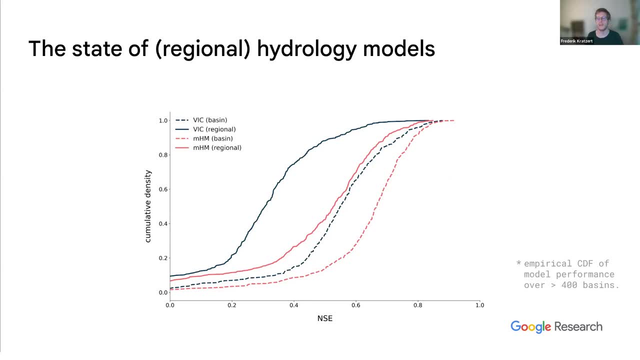 One model that is calibrated on all of these hundreds of basins together, And what we can see is that if we look, for example, at the median, which is the horizontal line, at 0.5,, if we then look at the NSE value of these different models, we can see that 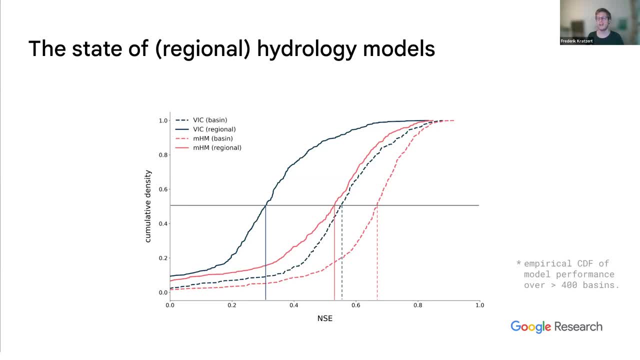 and that's true in all of hydrology- that the per basin calibrated hydrology model is much, much better than the regional calibrated counterpart, Even though it's the same model, it's just a different calibration scheme. So that's the first thing. 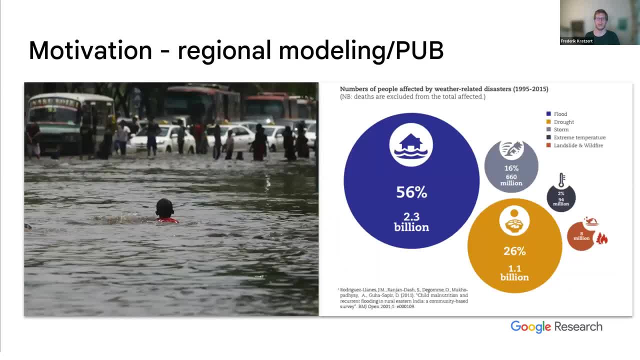 Thank you. So you might wonder why are regional models important? So this is actually a very good link to my work at Google. The reason- one reason actually- is, for example, flood forecasting. So floods are the number one most damaging and most dangerous natural hazard affecting 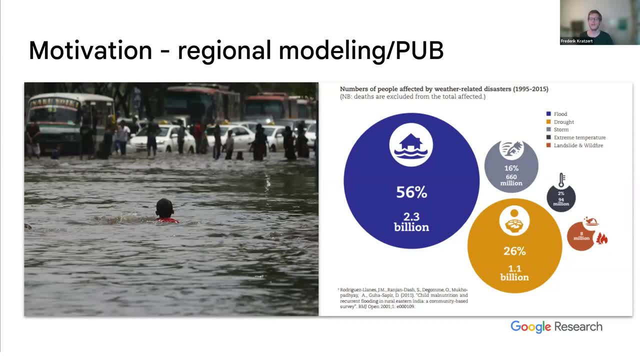 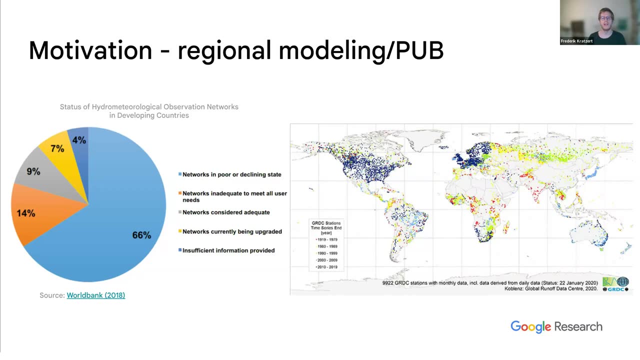 hundreds of million people every year. There are thousands and tens of thousands of fatalities and it costs more than 10 billion of economic damage per year. And the problem is that a lot of these very devastating floods occur in places where we don't have streamflow observations, or at least no recent streamflow observations. 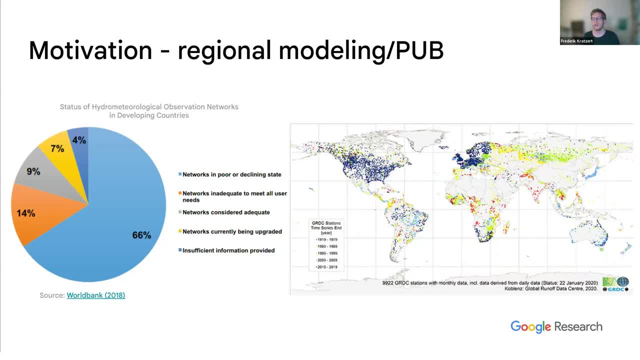 So actually you can't calibrate a model there. So we're in the position that we want to get flood forecasts in places where we don't have observations. So we're in the position that we want to get flood forecasts in places where we don't. 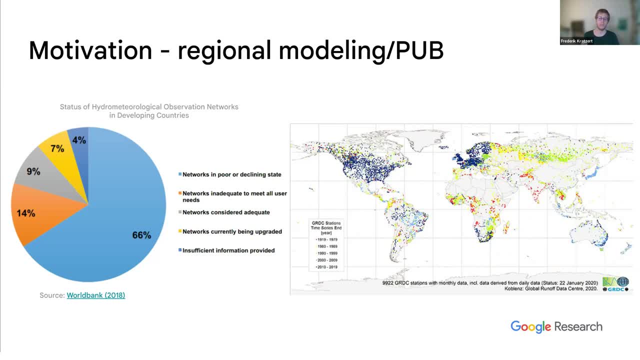 have observations. So we're in the position that we want to get flood forecasts in places where we don't have observations. So you can't calibrate a model that you're not raring to do, because we could prevent a lot of damage and save a lot of lives. but the models that we have are actually only. 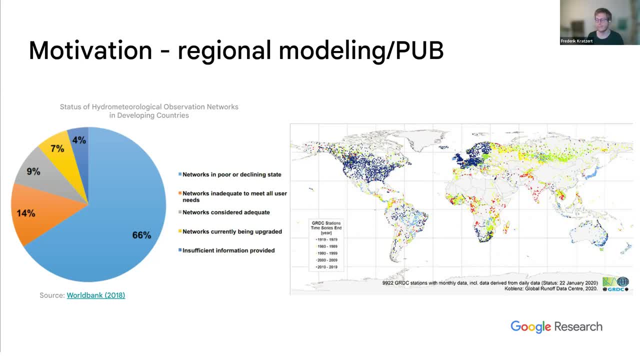 good if we can calibrate them specifically to each of the rivers. And it's actually not only a problem in low-income countries. Also in developing countries, the state of the existing gauge stations is declining, So this problem will become more and more severe over the next years and decades. 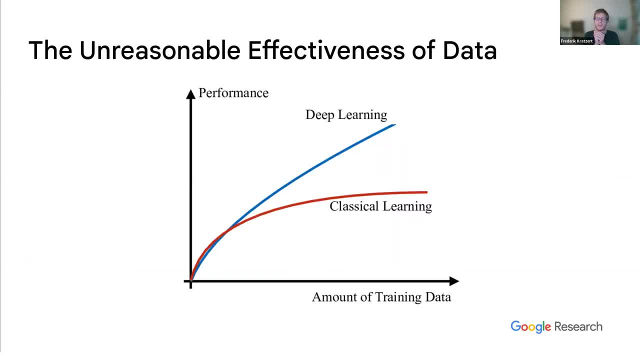 So we had the machine learning seminar, and getting worse with more data is actually, I would say, in contrast to what we know from machine learning. So when I started all of my research, I was still a master's student in hydrology, and 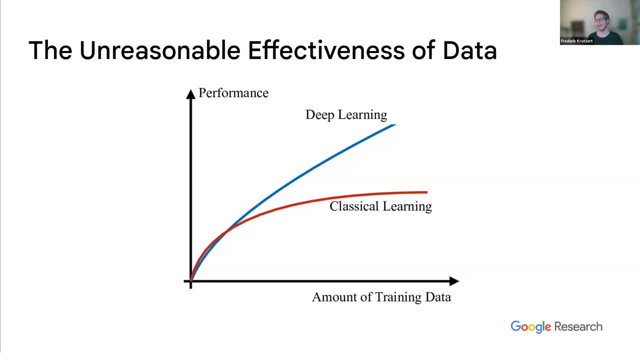 I was teaching myself machine learning and I would think: like wait, why is all of machine learning getting so much better with more data? and we in hydrology, if we train on multiple basins, on multiple rivers, we are getting worse, even though we actually could. 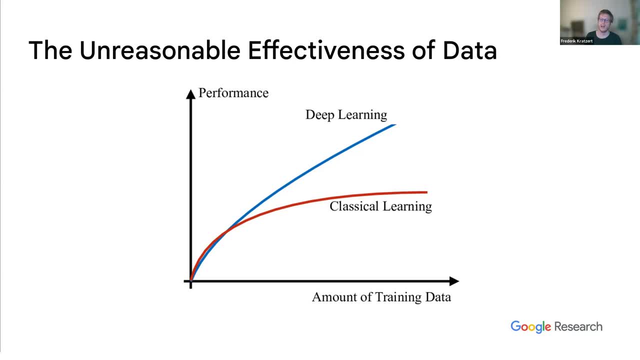 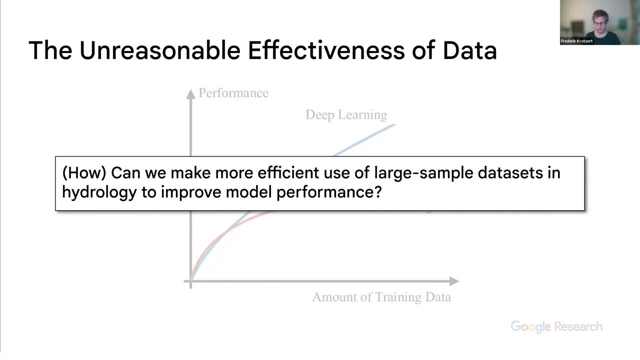 learn more about the underlying physics and processes. So the question I started to ask myself: how can we make more efficient use of all of these? because in hydrology we have lots of data. if we look at globally available streamflow data, How can we build models that actually leverage that? 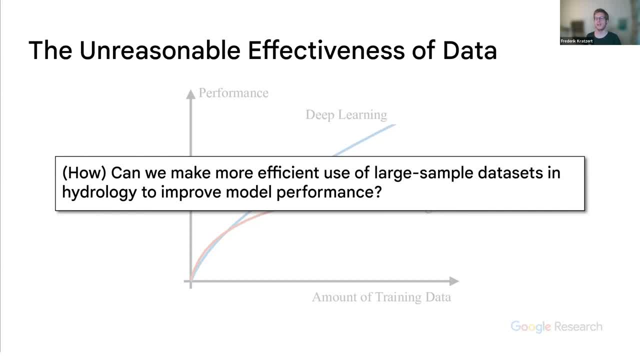 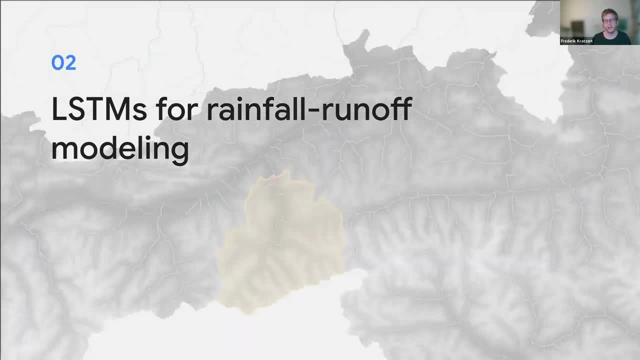 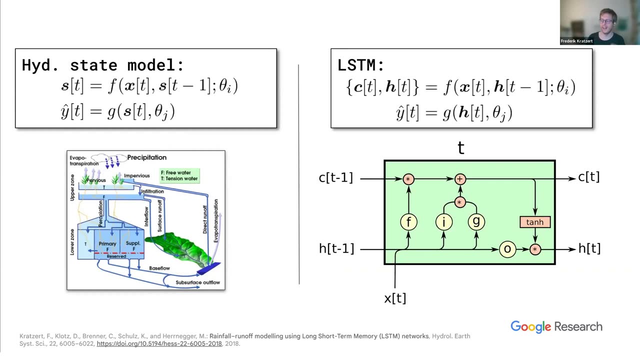 Leverage the data we have and can then get better at each individual location. So here's where the LSTM story starts. you might want to ask why using LSTMs? LSTMs are not used that much anymore today. So the question, the reason actually is- and I think until today they are still proven- 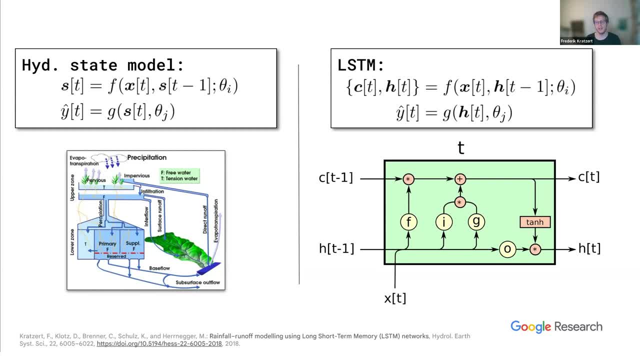 to be the best model for this application. The reason is that the LSTM is conservative. It's actually very identical to this underlying system that we're trying to model, and also to hydrology models actually. So I said before, we have these hydrology models that have that implement hydrological 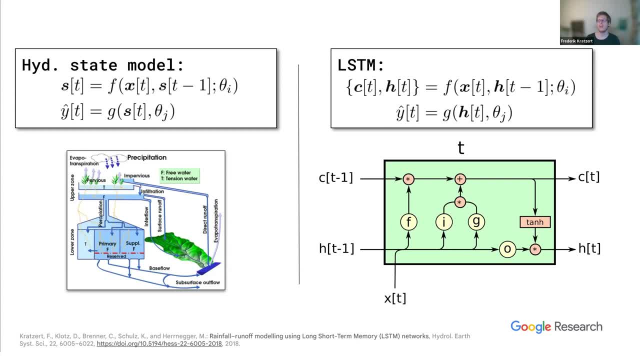 processes as states, and we can describe them as a state-based model. The states of the system are a function of the previous states, of the current inputs, and so model parameters, and the output is a function of the current states, and so model. 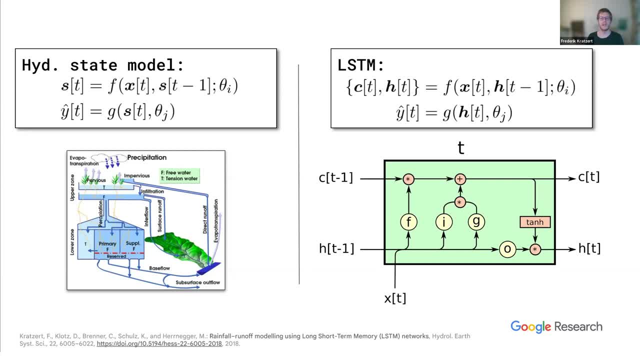 parameters, And this is actually exactly how we can define the LSTM. We have a state in the LSTM. this is also a function of the previous states- some model parameters that we learned during training- and the output is also a function of the current. 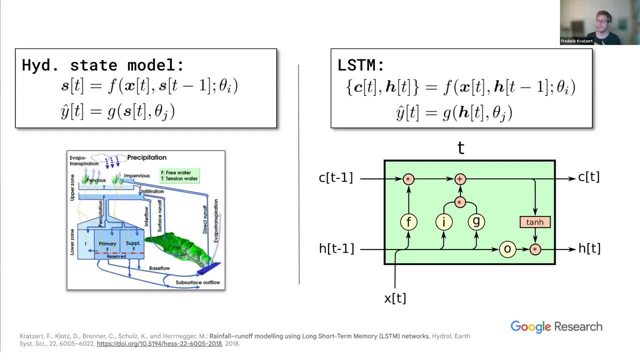 states. And actually, when I started to learn about machine learning and then there was a lecture about LSTMs and recurrent neural networks, I saw this similarity and I thought like, okay, let's try it, because to me it seems like the LSTM is a very good fit for the hydrological 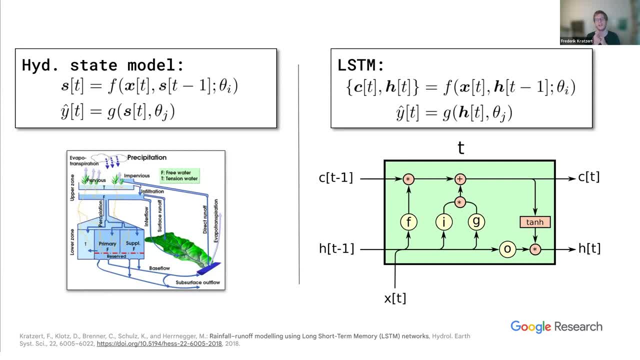 application, with the benefit that we don't have to decide upfront which hydrological processes are important in the catchment, which hydrological processes we want to include in our model, but we can let the model learn from data which processes are important. Now let's talk about the LSTM. 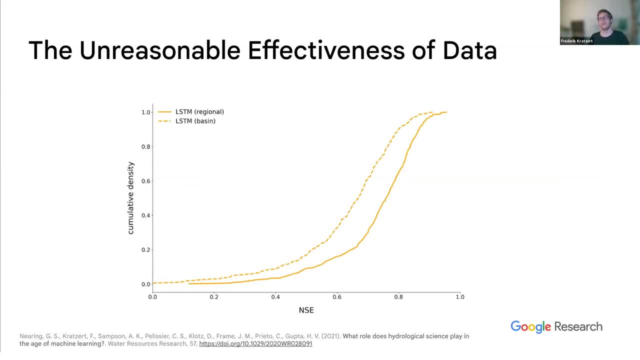 Let's talk about the LSTM. Okay, So I'm skipping. I'm not skipping, I'm jumping a few steps ahead and already tell you the difference of LSTMs compared to hydrology models, which is if you train LSTMs correctly. 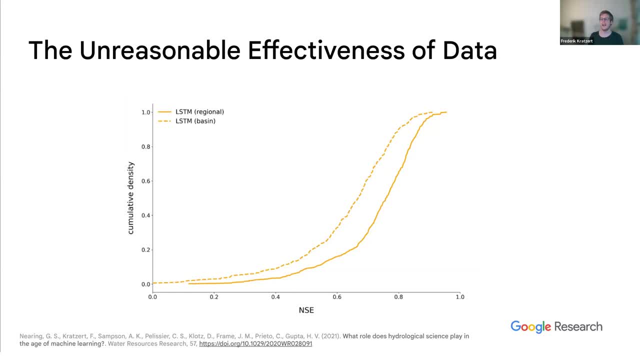 and I will come to that in a couple of slides. the LSTM is actually able to leverage information from being trained on multiple rivers and getting substantially better than if you train individual LSTMs. So let's talk about the LSTMs for each river and, yeah, we will look at what's the reason. 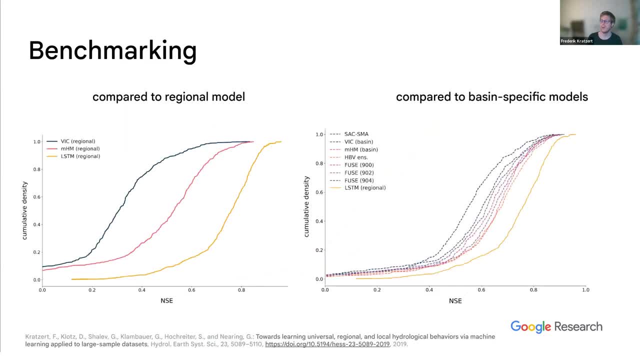 for that and how this works. in a couple of slides We can first look at how the LSTM compares to hydrology models and here, in all of these plots, the LSTM is always the yellow line. and again, this is the CDF. so the better. 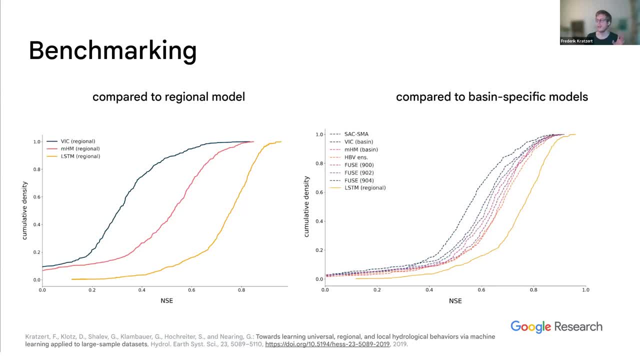 model, the further to the right is the line. The left plot compares a single LSTM, One LSTM. It was trained on the same hundreds of basins, on the same period, with the same inputs to regional hydrology models, which is actually the fair comparison, because the LSTM was 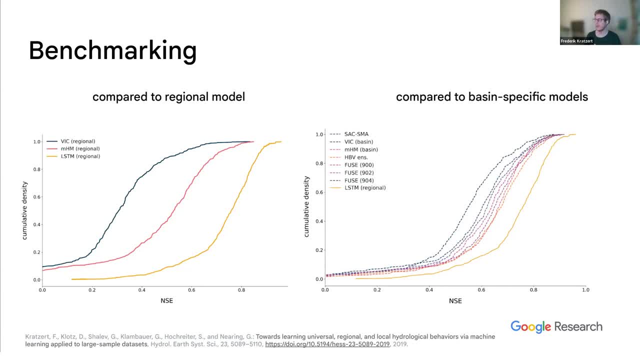 also trained, let's say, in a regional fashion. And the right plot with dashed lines compares the LSTM to different single-basin calibrated hydrology models. All of these models were calibrated by different researchers, most of the times by the model. 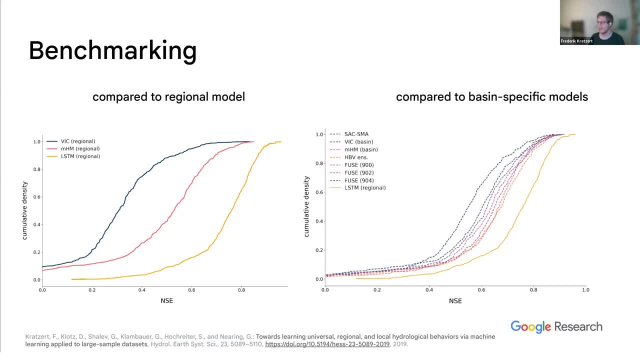 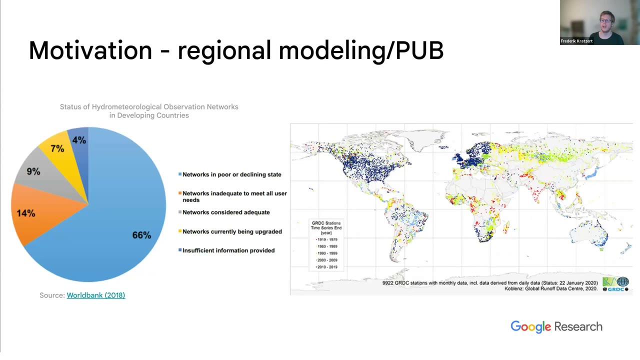 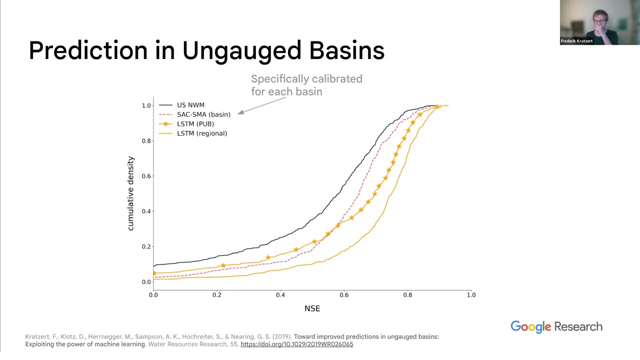 developers themselves, So they should be fairly good calibrated And we can see that in all of these cases, the single LSTM being trained on data from all rivers is better than what we had in hydrology so far. Sorry, these slides were there. 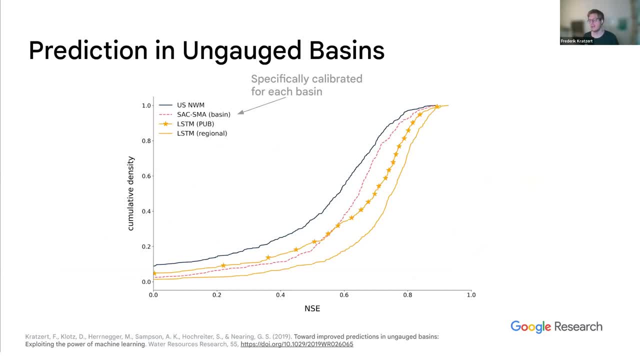 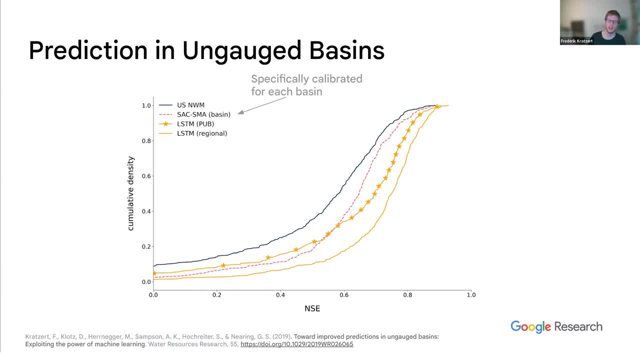 How good is the LSTM? How good is the LSTM? How good is the LSTM? I think the LSTM is very good. The most critical part is the LSTM actually predicting in rivers that were outside the training data, Because one of the most heard critiques I got at the beginning of my PhD from the hydrological 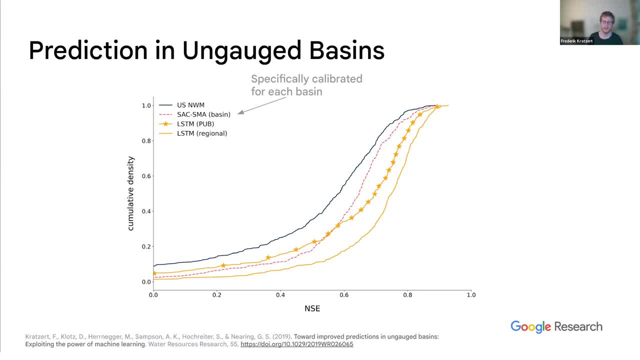 community was that LSTM's machine learning models only fit in training data. They are not being able to generalize to unseen rivers. They don't understand the system, all of this. So I said to myself: one of the best ways to do this. 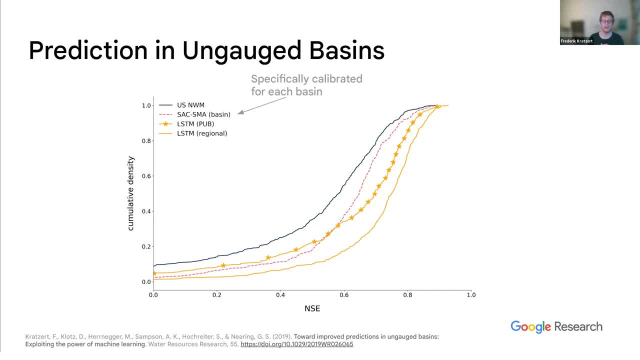 Okay, Thank you. to test it is to hold out a set of rivers, train a model of all remaining basins and then see how well does the model perform in what we, as a project call un-gauge basins, This actually even more stringent tested. 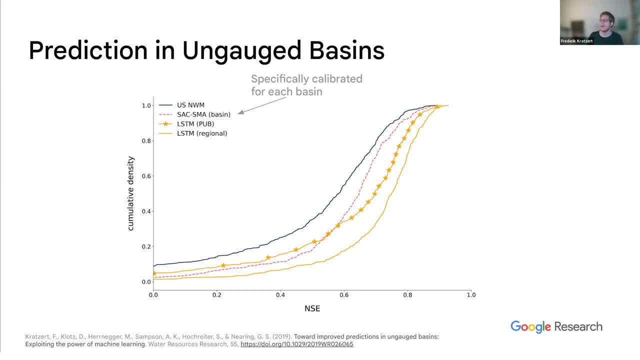 the better test for what we at Google currently are doing. So what we see in this slide is the LSTM from the previous slide being just the yellow solid line, compared to an LSTM that was trained on a k-fold cross-validation, with always keeping one fold out. 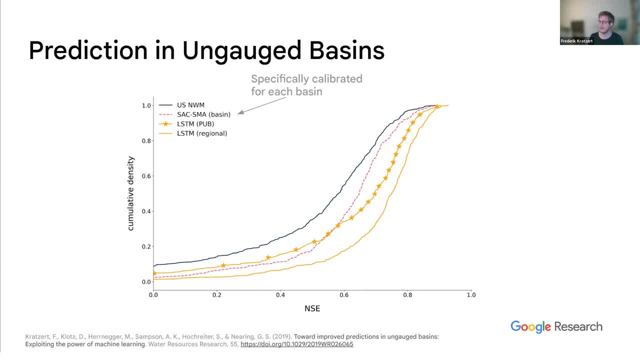 and training on the remaining folds and then validating on the holdout basins set, which is the yellow line with the asterisk markers. And then we have two hydrology models here for comparison. Both of these models were calibrated for all of these rivers. 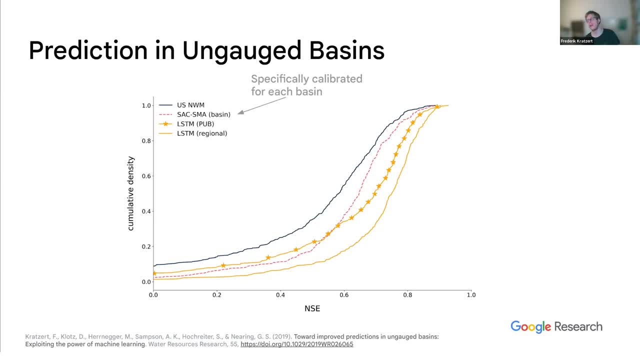 So we have the dashed line, which is the Sacramento model, which is like a benchmark model being part of the data set that I use. So this is actually an ensemble of 10 models being calibrated for each river individually. And then the solid blue line. 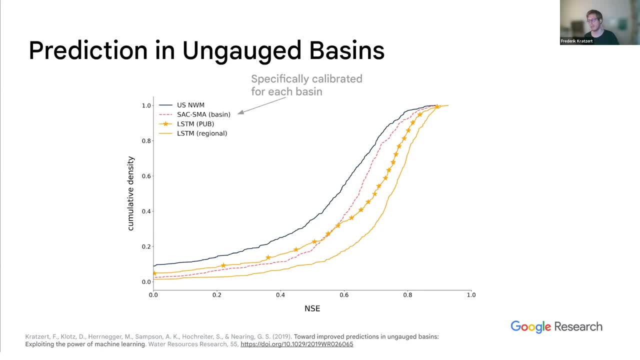 is the current US National Water Model, which is now being deprecated, but it's still the operational US National Water Model which is also calibrated for most of these stations, And we can see that the LSTM is actually better in giving predictions in the majority of the rivers. 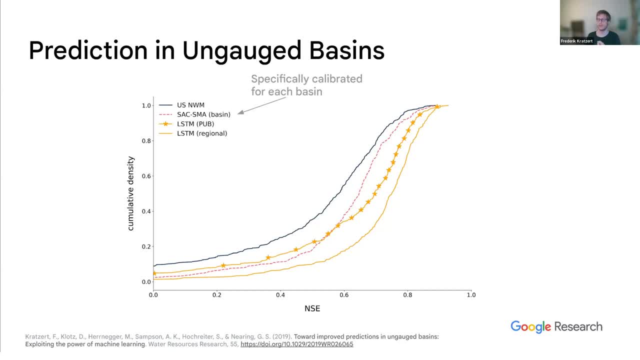 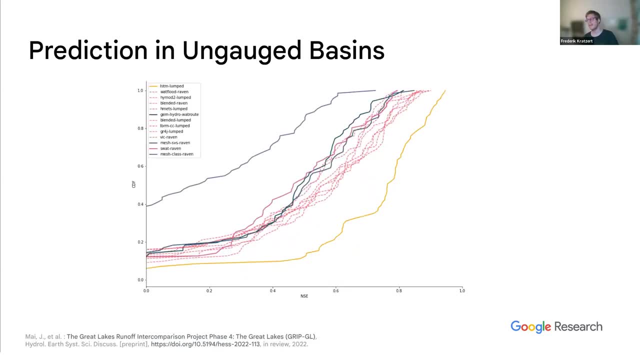 than a hydrology model that was calibrated for all of these rivers individually And from a very recent study where we had a test. so this was a challenge where we participated from Canada, and there are Canada, the US, actually from the Great Lakes region. 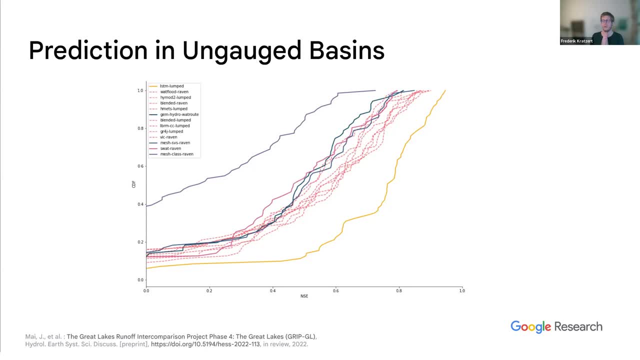 So there was a model inter comparison study where each group that participated got only the training data and for the validation period, We got only data. So there was a great challenge in terms of the data and for the validation period, we got only the training data. 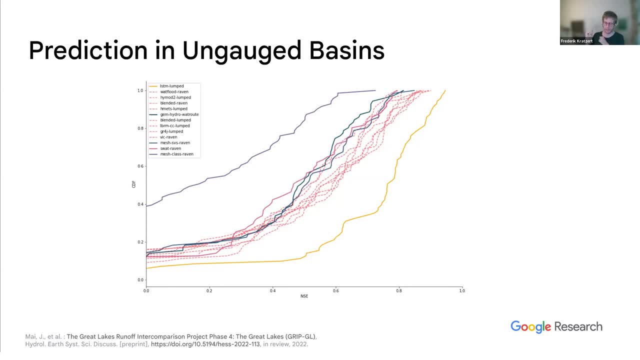 So there was a great challenge in terms of the data and for the validation period. we got only the training data, input data to the model and we had to provide model simulations. We could only provide the model simulations once. We could not write a sheet by knowing our score and then trying to recalibrate. 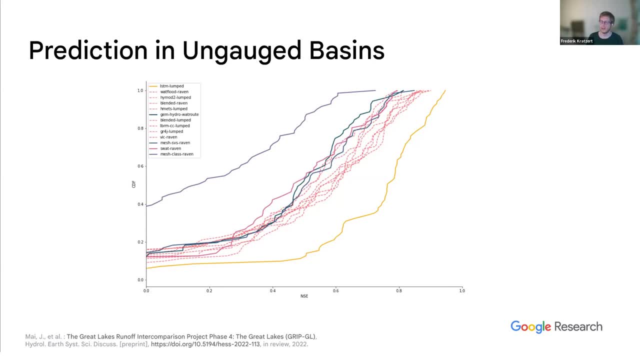 or whatever. So a lot of groups participated and some of the models that you see here were also present on the previous slide. So this is actually a comparison again of prediction and angage basins of the LSTM and all of these other models predicting discharge in rivers that. 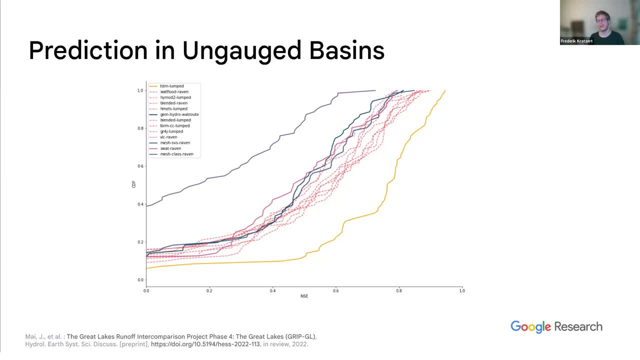 they were not trained for. We can actually see that the LSTM is quite good in predicting and angage basins, which can only happen if it understands the underlying system and if it is like understanding the processes that drive the river discharge. So a question in this? Yeah, sure, So could you say a couple of words of how the traditional 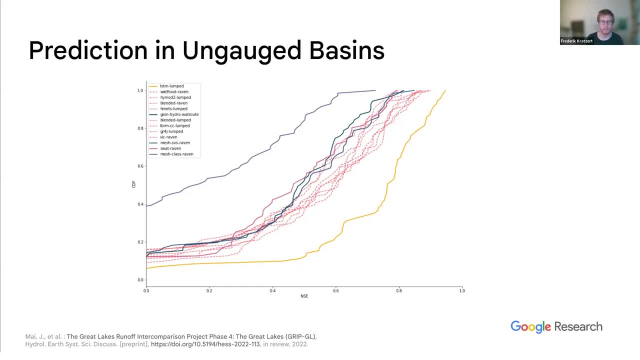 hydrology models are calibrated. How is that process carried out? Yeah, so these are mostly non-differentiable models, So they use various different calibration methods, ranging from genetic algorithms. I think that the most common optimization strategy is used as a DDS algorithm. 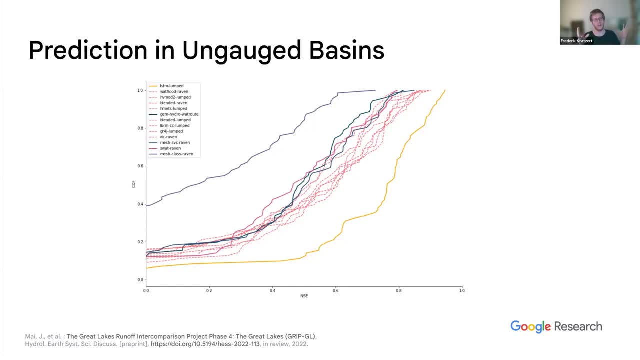 So, but basically it's like generating a set of model parameters, doing inference in the models, seeing how well each model parameter set fits, and then adjusting the model parameters. So yeah, not by differentiation. Yeah, so that takes time. Yeah, so that takes time. Yeah, so that takes time. 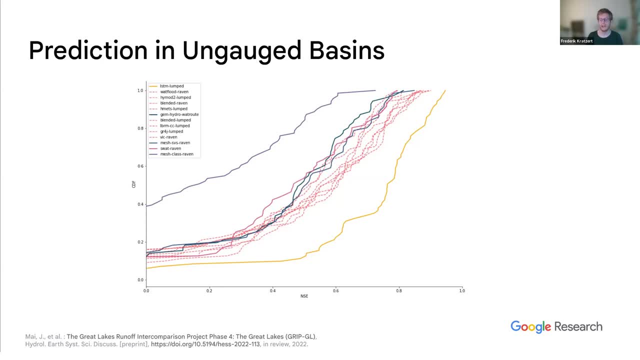 Right, So actually that's a very good point. Initially, hydrologists often claim that training deep learning models requires a lot of compute and it's quite time intensive. Calibrating hydrology models on the same set of hundreds of stations takes months. We have training in LSTM, I think most of you know, on like. 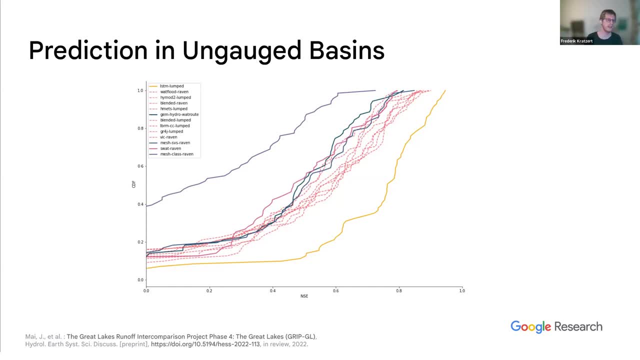 I don't know. a single GPU takes a couple like with this. data set size takes like two or three hours, So it's the other way around. It's like much more expensive to calibrate hydrology one, even though doing inference on this model once is like super cheap because it's like fortran code most of the. 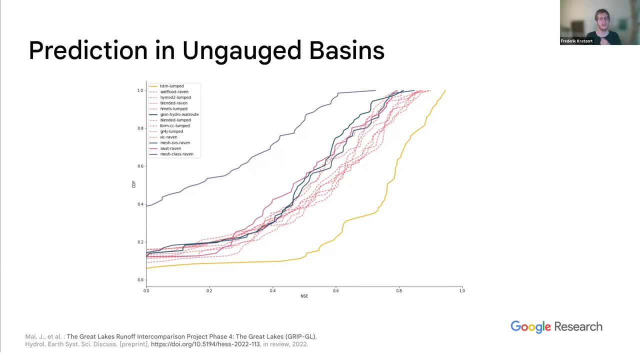 time There's like no magic happening, but then calibrating them is usually it was like thousand and hundred thousand so far. Thanks, Anymore questions? No, okay, So the next thing that we will look at is how does it actually work? Like, how is the LSTM? 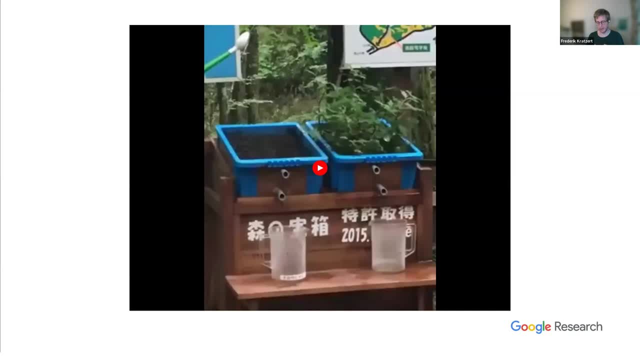 being able to, to learn from, like a large and diverse set of reservations and then being able to with like predictions. And yeah, a couple of years ago I found this video. unfortunately it was on the videodump home page and I don't know the lem: você également acutuamente tem uma filha. 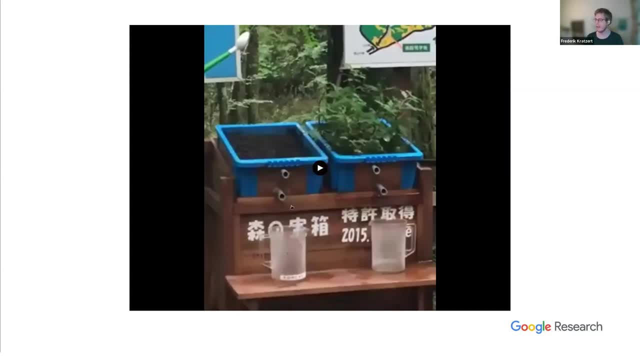 ici de uma base de vídeo. I don't know the site, of course, but on the website, of course, I can actually find the code based on that article. i don't know the source. it must be, i think, from chinese university, probably a research unit. so what we see here, i already start the video. it's like um. 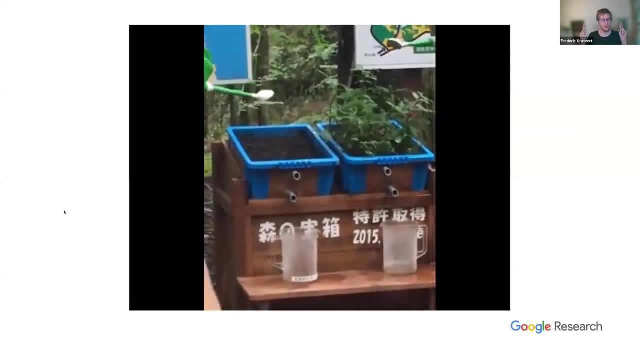 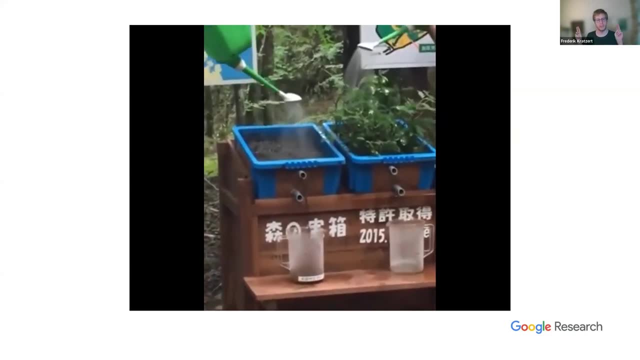 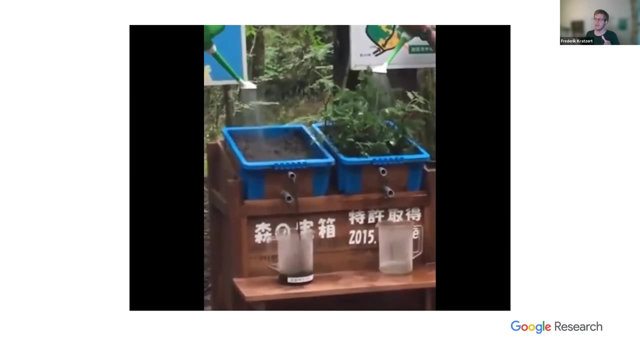 you see two boxes. so these two blue boxes represent two catchments, two basins. both have the same shape. they get exactly the same meteorological forcings, being like the room temperature and the water being applied to them. they have the same slope. the only difference is: 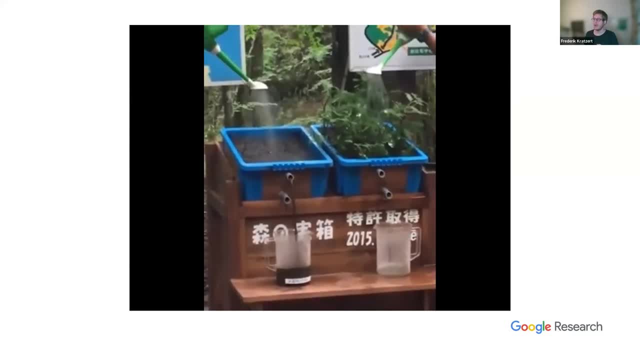 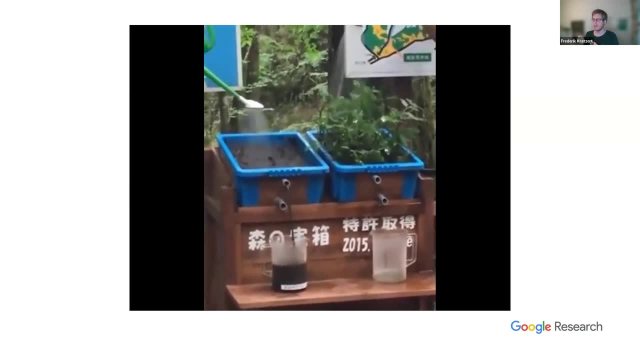 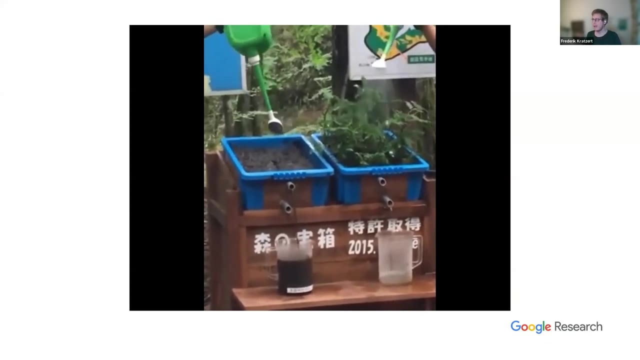 the vegetation in the boxes right and you see how the difference in the vegetation in the boxes decided in completely different response from the attachment. so the one without vegetation is immediately like draining all the water, very muddy, into the glass and while the left box is already like finished draining its mercury water, the right 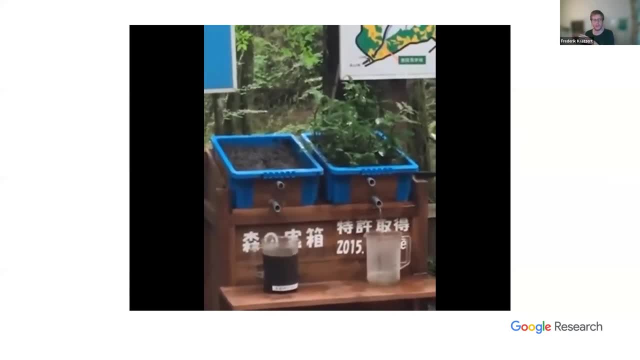 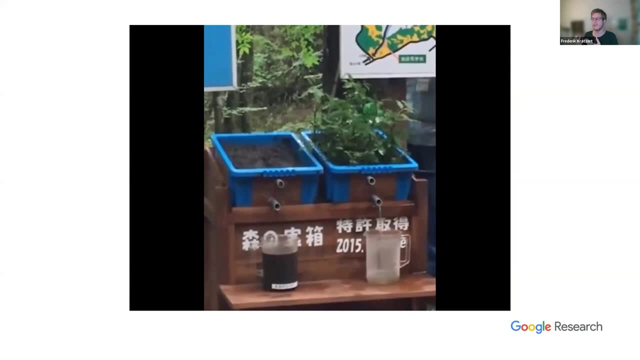 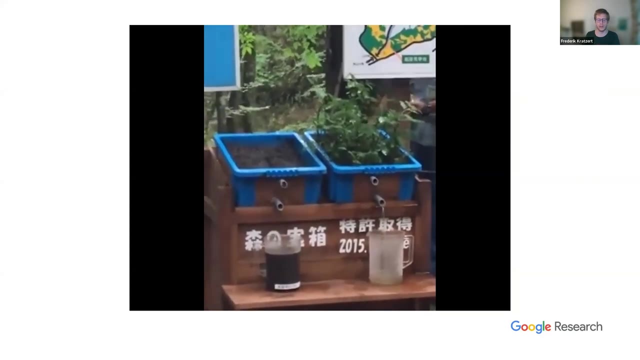 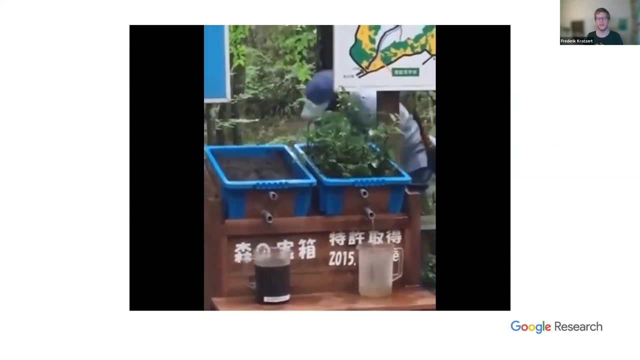 box is just starting to drip water from the lower tube, being very clear water. so the only way our model that has to model both of these boxes and gets us input, metrological forcings, which is like the usual input in metro hydrology models- is able to learn how the boxes should like react, is if we 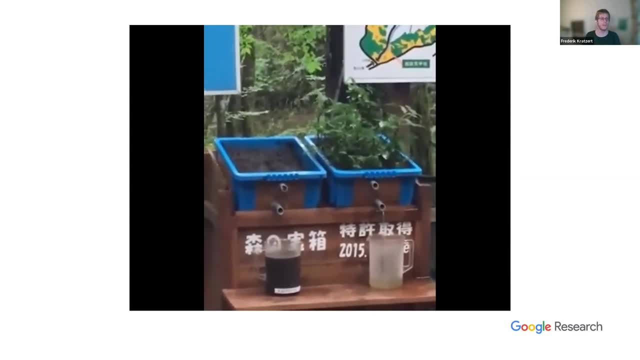 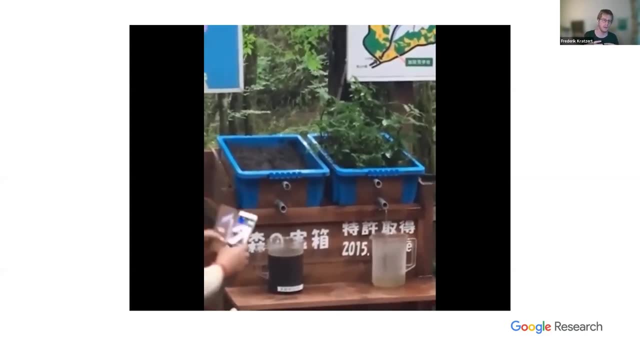 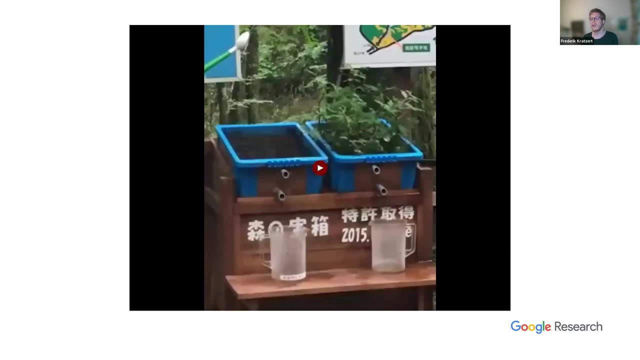 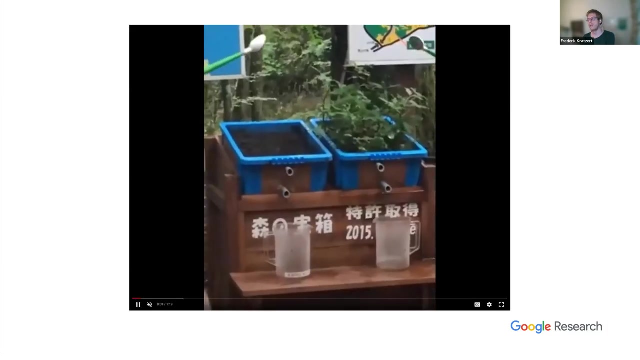 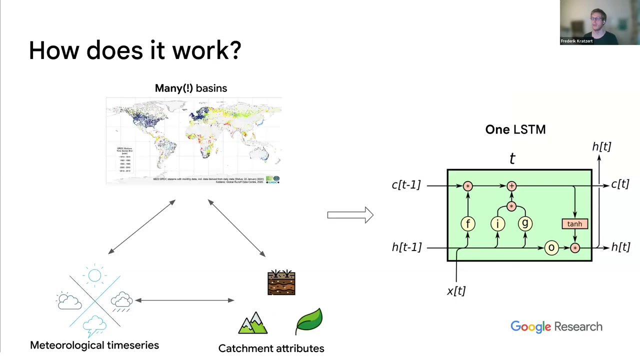 provide additional, like static catchment attributes or some additional information that box a has no vegetation. box b is like a dense forest that absorbs a lot of the rain and like buffers. the response: so this is exactly how it works, and which is sorry. i think it should be 521, right? so this is exactly how it works, what we do, and this is also true for 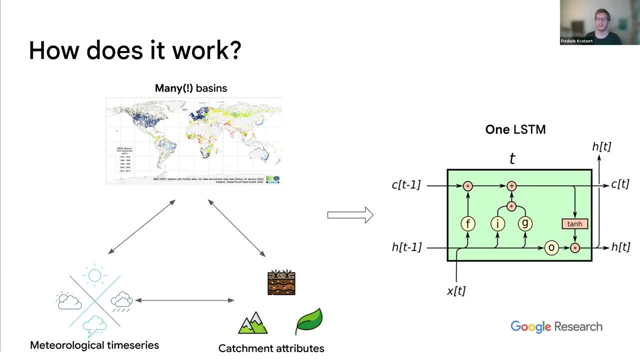 here at google. what we do is we take this charge data from all around the world, we extract metrological time series for the basin area- and the more different metrological products the better- and then we also derive catchment attributes, and these are things like the elevation, the topology. 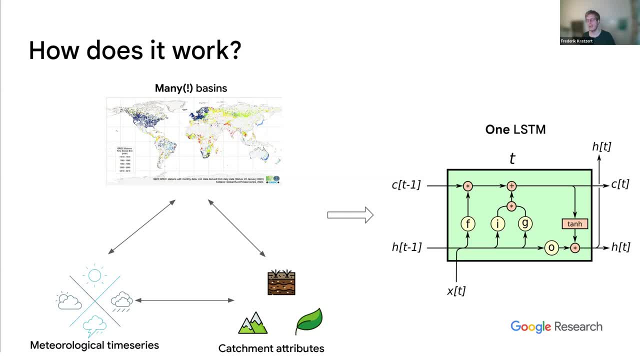 the slow vegetation, information about the soil, long-term climate, ind outward climate ili se anything to inform the model it is now giving prediction in, i don't know, a mountain catchment or in an arid catchment or whatever you want. this is encoded on the catchment attributes. 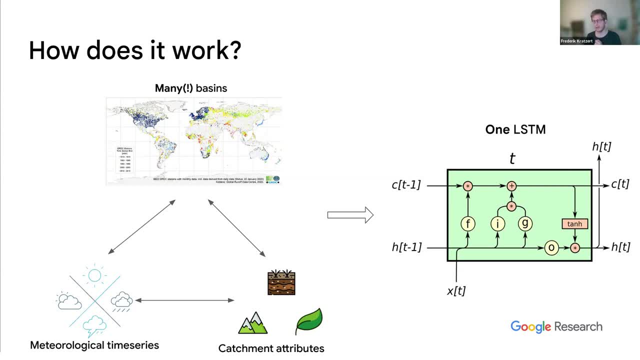 and then we train a single LSTM and one input set into the LST is a time series of metrological data, the catchment attributes that correspond to this one catchment, and then the target data is the discharge for this one. basically, And this is all the magic behind the model, actually, 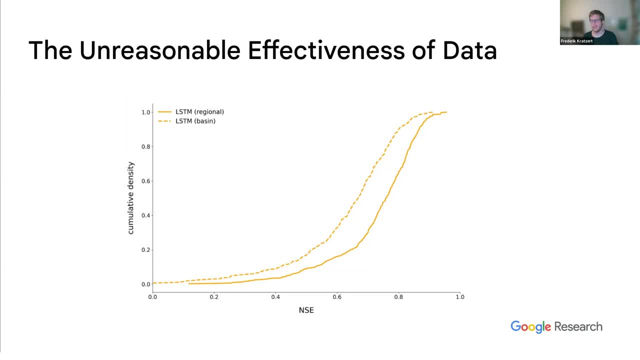 Now being done with how the model works. I have two different ways how we can continue with this presentation. One is work on model interpretability- that I spent a considerable amount of time in my past to look at what the model actually learns about underlying processes, And another one is: 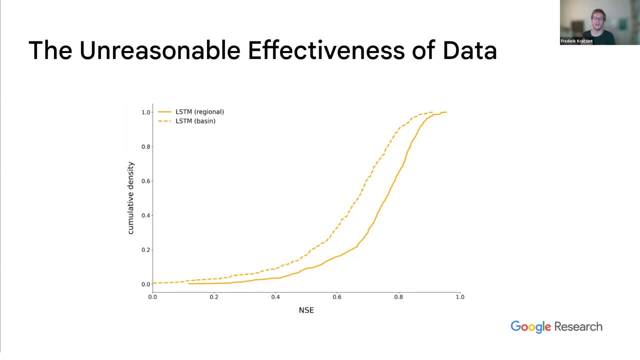 one that I like to talk a lot about, which is why you should never train an LSTM, actually for a single river. What HydroGIS used to do with the hydrology models, the best thing they could do is to train a model for each river individually. While it was LSTM. there was LSTM to do the test by hand. Anything else you want to add in the feed? Food and beverage. Anything else you want to add in the feed? Yes, Let's just go ahead. Would you just get the video on line then? 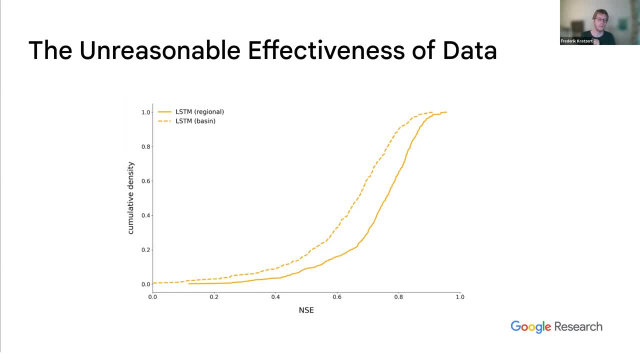 LSTMs. you should actually never do this like not only is it worse, but it has certain problems, and I don't know if we can like make a use the chat and I give you like 10 seconds and you write A or B, and if you write A, we will do model interpretability. if you write B, we will continue. 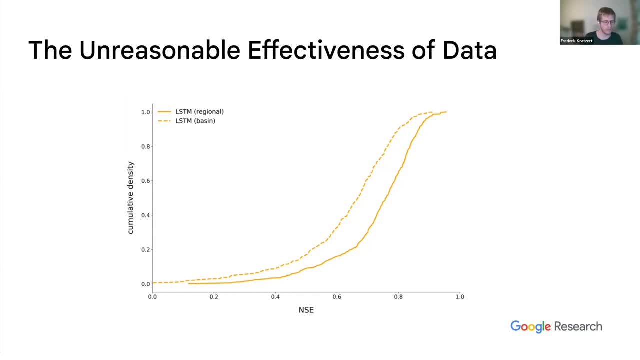 with why you should never train a single-based LSTM. let's see if we get some replies. I will take the majority vote. so A is interpretability and B is never train a single-based in LSTM. okay, I'll give you like 10 more seconds. okay, I'll stop here. I don't count for the double votes. 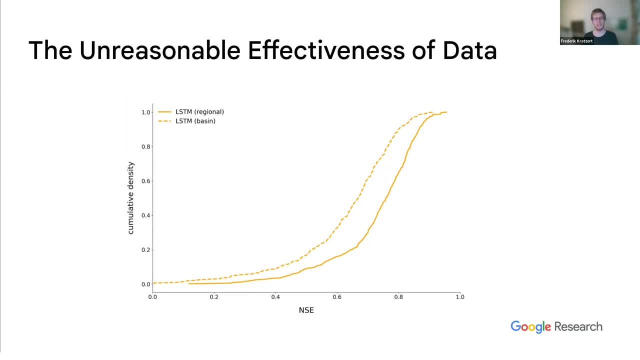 one, two, three, four, five, six. okay, I think B won with. B was the why you should never train a single-based LSTM, if I read that correctly. okay, so the point here is that LSTMs- like I heard and talked earlier this week, actually that in almost 50 percent of all hydrology papers that are published now, LSTMs are actually being 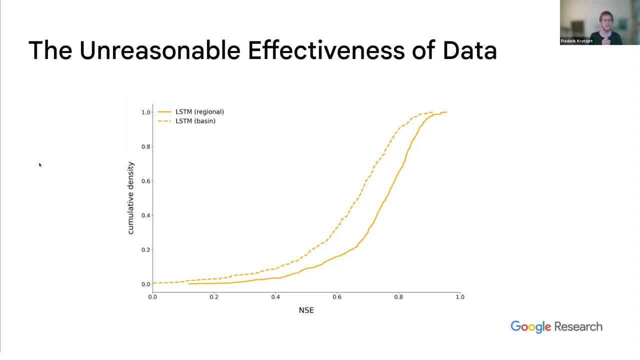 discussed. either they are being applied or they are being discussed in their introduction or conclusion, but LSTMs became very popular in LSTM over the last years. the problem is that that's my opinion. I hope I can convince you that it's correct that hydrologists tend to 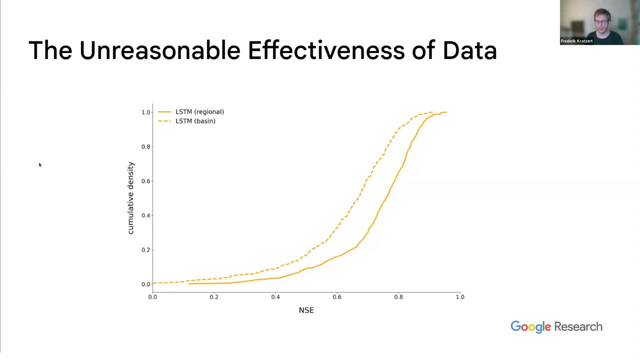 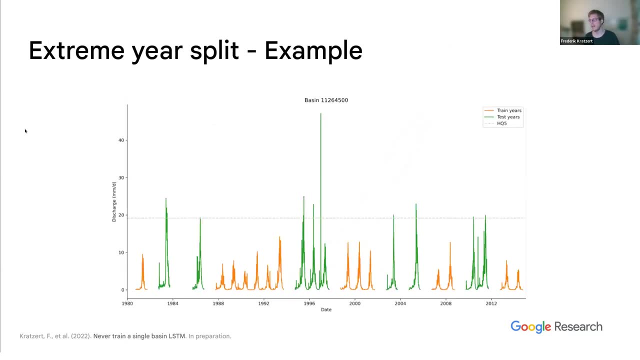 apply these models incorrect. so- and the audience here is mainly machine learning, so this might not be a surprise- Flap year flood, five year flood and is what statistically should happen once every five years. okay, This is like a measure that we use for return periods, how we can characterize floods and being severe floods or rare floods or whatever. 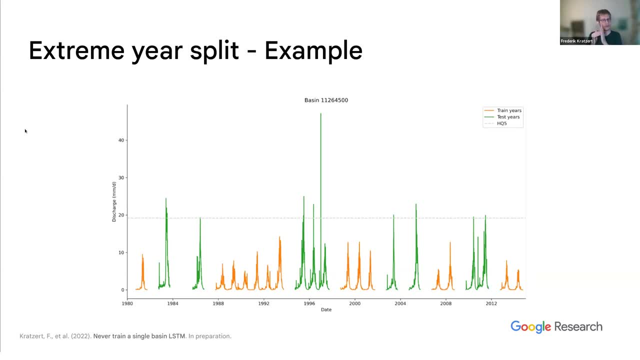 So we take all the years where the flood is below its threshold- like the maximum annual discharge is below its threshold- then we use this year's training data. If the maximum annual discharge is above the threshold, we use it as test data And then we take all these training years again from all of our hundreds of basins to get a training model on this. 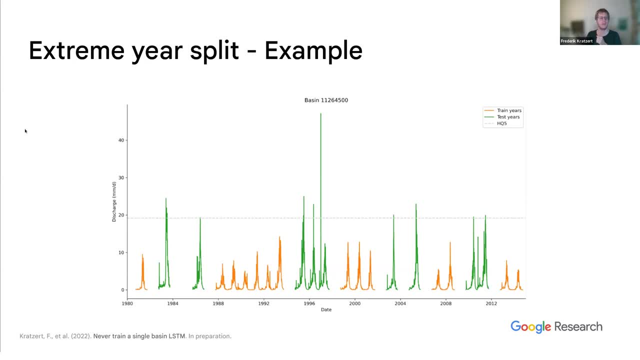 versus training models individually for each river. And remember that these rivers are completely different, So they have different discharge magnitudes. So what is like a H2O, like a 20-year return period, in one basin might be a very normal magnitude of flow in a different basin right. 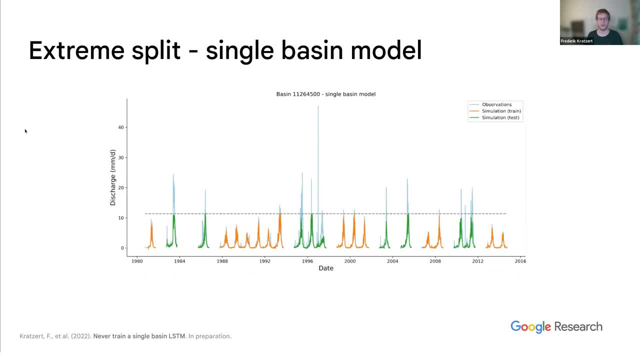 So what happens if we train a single-basin model that only sees the data of one basin? So if we train a single-basin model, I think all of you that have a background in machine learning will know that you are probably not able to predict anything that does not occur in the training data, right? 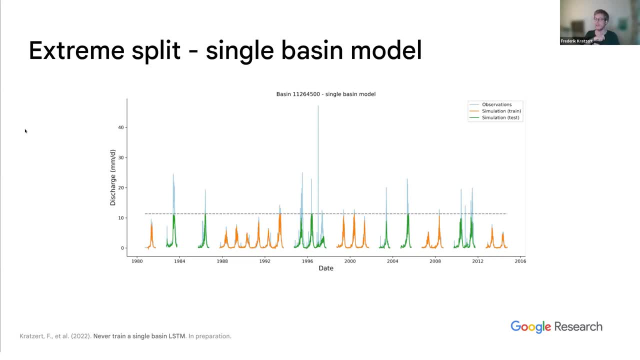 So what you see here is now in blue, in the background, you see the observation. Orange is the model simulation of the training period. So this is actually the training data. It's like fitted to this data, and then the simulation after the model was trained. And green is the simulation of the validation period. 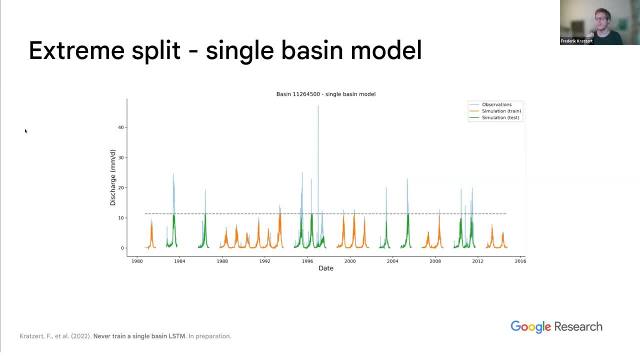 And the dashed line that you see is the maximum of the simulations of the training period. So it's the highest value that the model was able to output during the training data, And what you can see is that it is basically not able to predict any value higher than this threshold in its test data. 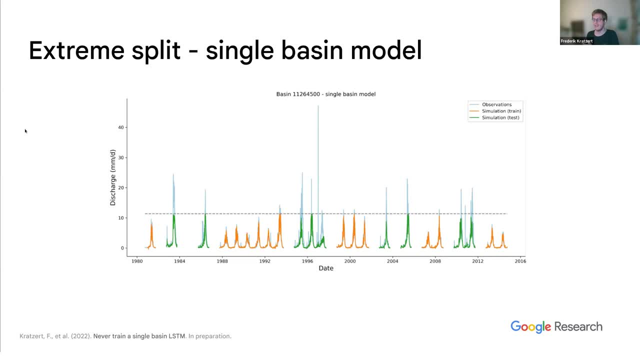 Which I would say it's no surprise, right? It's like the model has never seen anything larger than this. The LSTM has a couple of saturation functions, It just doesn't know. Probably the precipitation input is much higher than anything it has seen during training data. 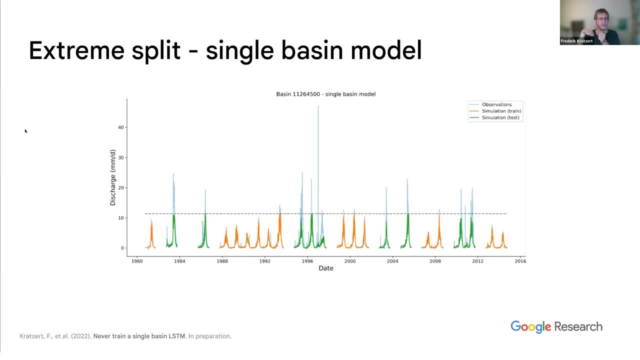 And this would just diminish in the input activation functions of the LSTM. So, anyway, you get this picture Now, if you train an LSTM on the same data split but you train like a regional LSTM, again being one LSTM being trained on hundreds of basins with 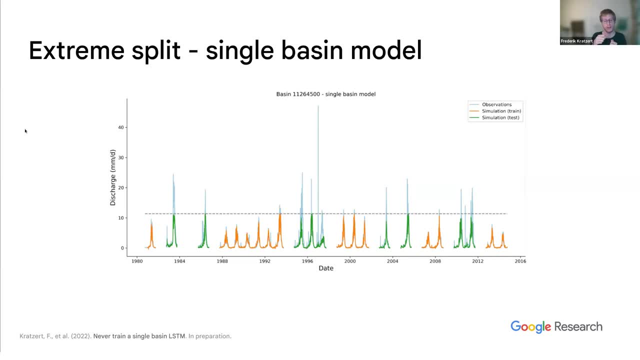 additional static attributes to inform the model of the different kinds of catchments, and then also the metrological forces, you get this picture. So what we can see here is that the model is actually able to consistently predict values higher than that maximum training simulation of this one basin right. 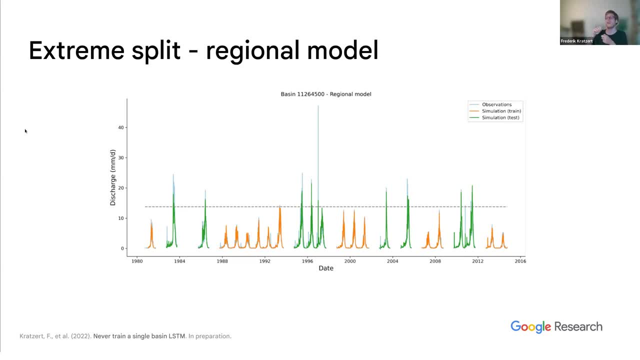 So that horizontal dashed line is the maximum discharge amount this model was able to predict in this basin during the training period And then in the validation period it sees higher peaks. And again, why does it happen? Because it has seen a couple of flows that are much higher in magnitudes in different basins. 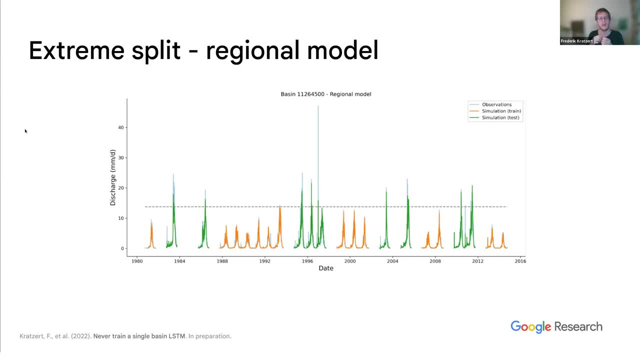 And because we train a model on all of this data together, we inform it on differences and similarities between attachments. it is able to transfer this knowledge into this basin. so it doesn't have the saturation point As an asterisk here. it still has the saturation point, but only in the basin with the absolute and highest discharge. 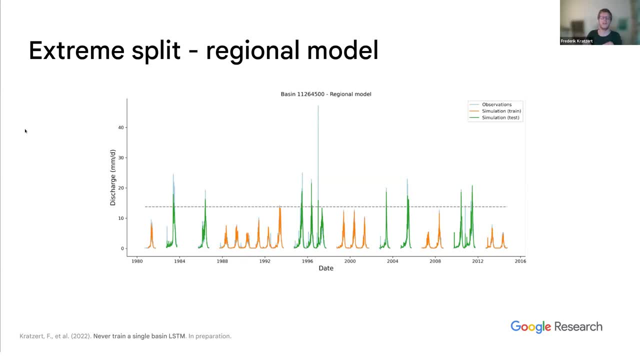 There the saturation still exists. But in all basins where flows are below this threshold, like below this maximum observed discharge during the training period, we basically don't observe any saturation in the model at all. In fact- a fun fact in our data that we have in Google where we train on a couple of thousand stages there- 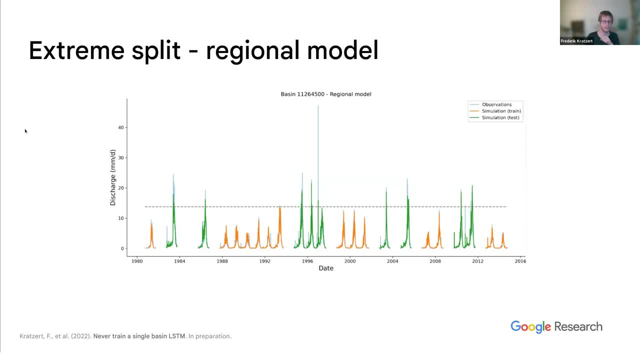 we have a handful of stages that have significantly like individual peaks that are significantly higher than individual basins, Anything that happens anywhere else in the world, And these- I think it's really five- these five stages raise the saturation threshold that high. 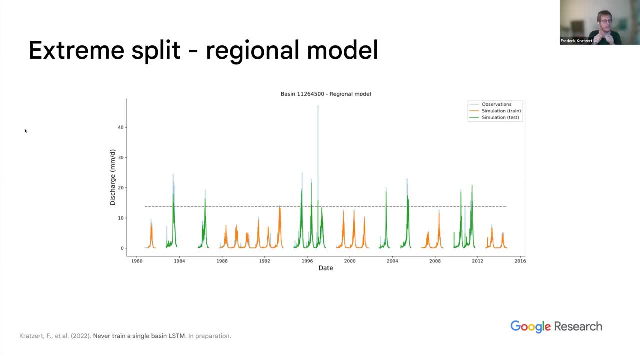 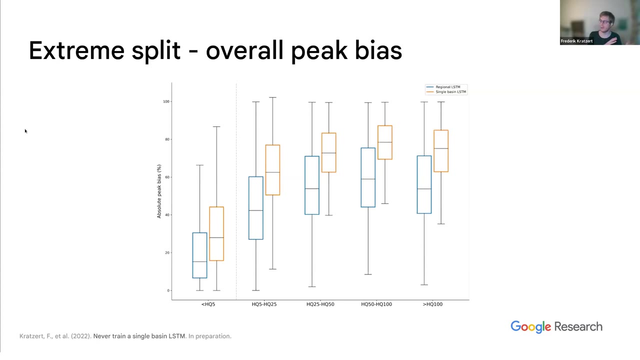 that in 99.9% of our stages we never hit the saturation point of the model. So here's the evaluation of these two different sets of models: the regional model in blue and the single basin LSTMs in orange. 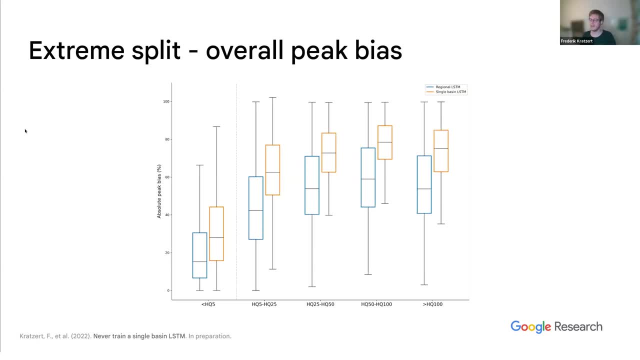 Over different flood peaks. We don't need to go into the details here. The thing that this figure should tell you is that, with higher or lower probability, floods being like the HQ5 as a five-year return period, the HQ25 as one flood that statistically appears one every 25 years, and so on. 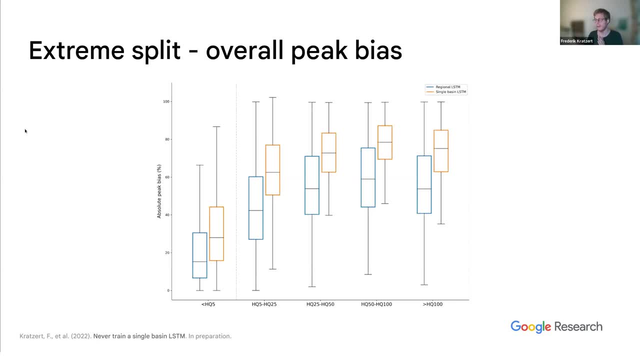 So the further to the right, the lower the probability of an event. The error of the regional LSTM like is consistently lower than the single basin LSTM, which is just what we have seen in the last slides. The difference that I've shown initially of the NSE, like the air squared between the 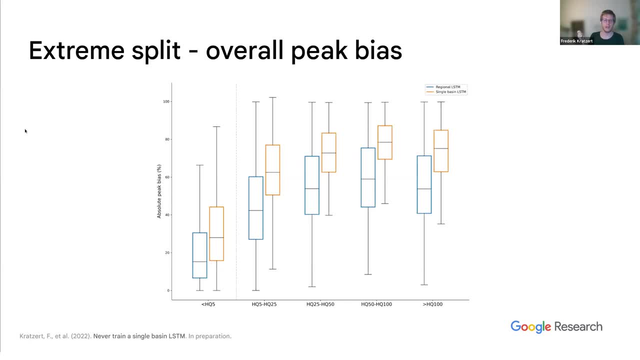 simulation and observation is not only explainable by the peak flow differences. The regional LSTM is better in any metric than the single basin LSTM That we usually evaluate models on. So it's also better in low flows, in mid flows, in the timing of the peaks. 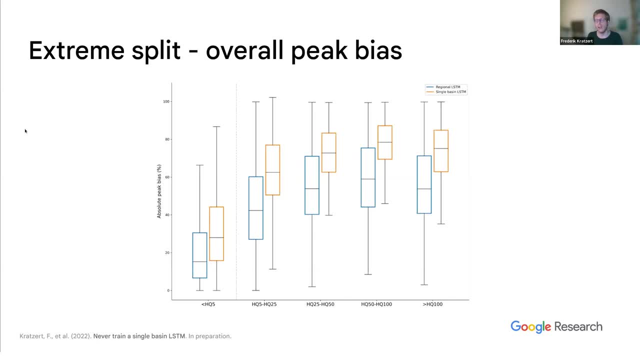 So the model is really getting like a lot out of being trained from the river, And not only that, it's better to predict the peaks. So there's a question on chat. Yes, What should be prepared? Train data should be based on threshold or simply split the time series as number of years. 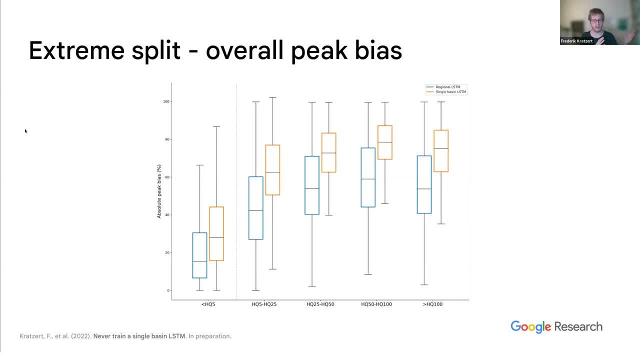 So definitely like train the split on the time series. What I did here was to do the extreme, just to like demonstrate the problem of the situation. Ideally, you train the model on as much data as possible and include as high as peaks as possible. 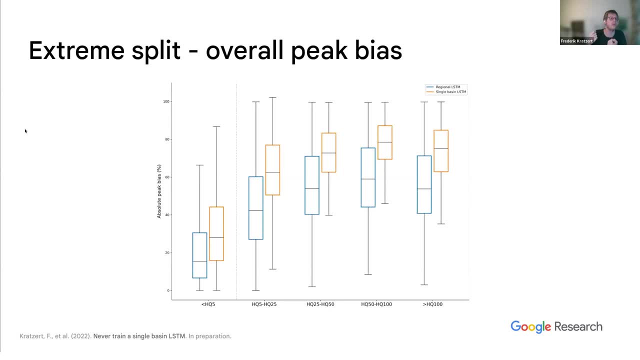 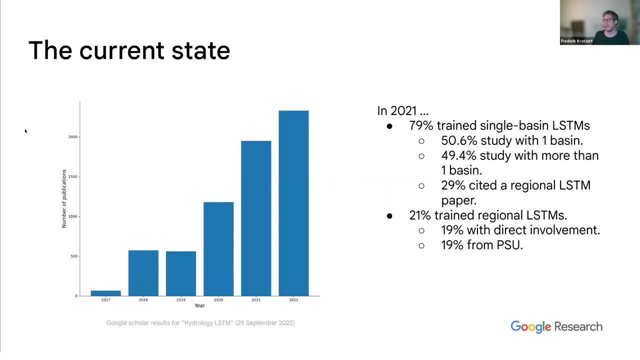 At least in our application for flood forecasting. we certainly want to include a lot of high peak floods also in the training data. So this is what I mentioned initially. We did like a literature research on recent publications in hydrology, all being published in 2029.. 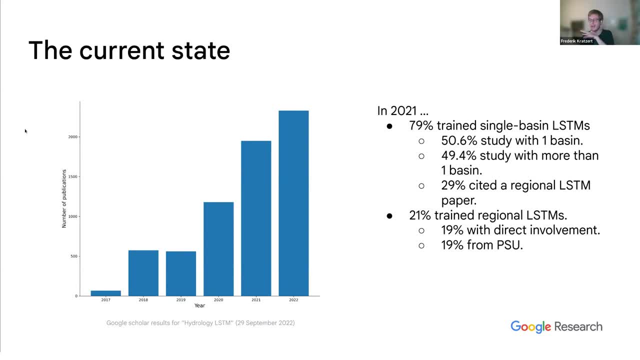 So the bar plot is just publications mentioning LSTMs over the last couple of years And from, like a literature research that we did on papers being published in 2021, around 80% of the papers applied the LSTM as a single basin model. 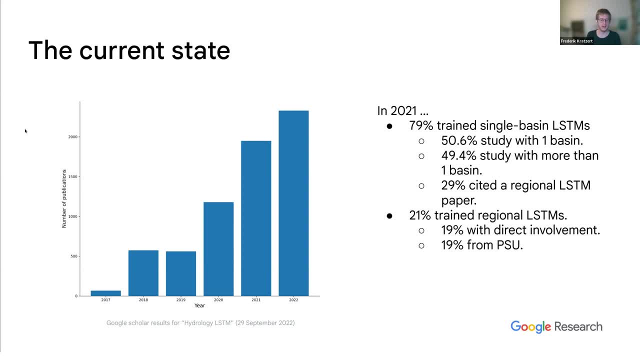 Again, and this is no surprise, because this is the state of the art, the best practice for any hydrology model. This is what hydrologists have done for like the last decades, actually forever. So the very standard model setup is taking one basin and comparing two different models. 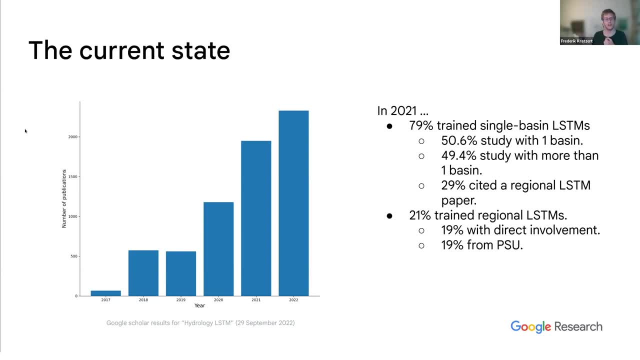 And now because everybody starts to use LSTMs. what hydrologists do is just apply the LSTM the same way and then getting good or not good results And, yeah, only a small fraction of papers actually doing the regional model stuff. 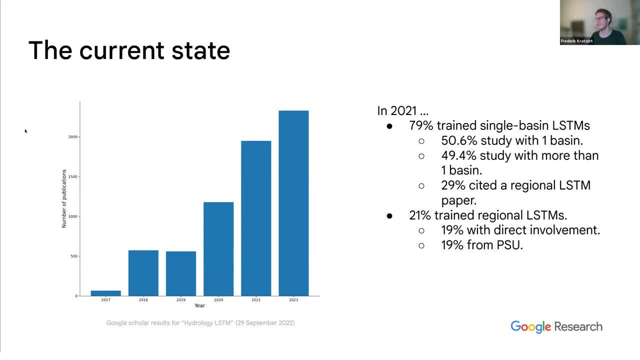 of which, like 20% of these, 20% of 20% are papers from, like, my group and colleagues, And the other 20% is like a group from Penn State University which is also publishing a lot in this direction. 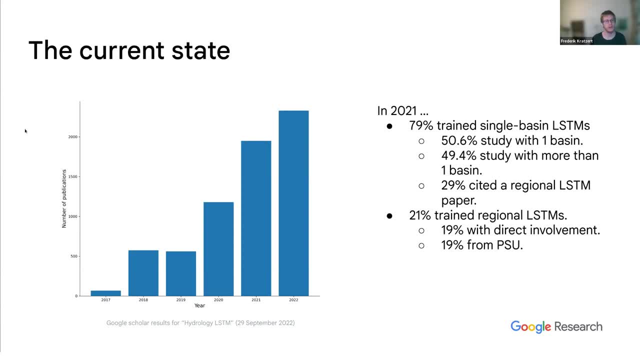 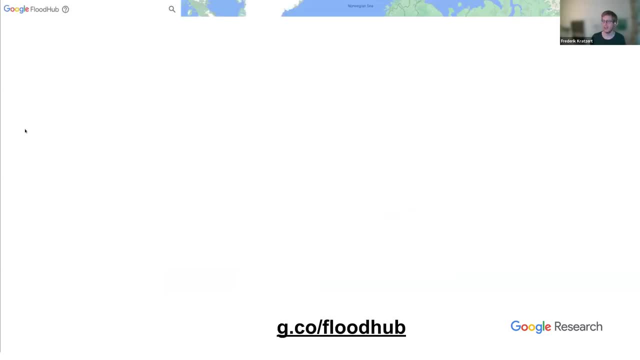 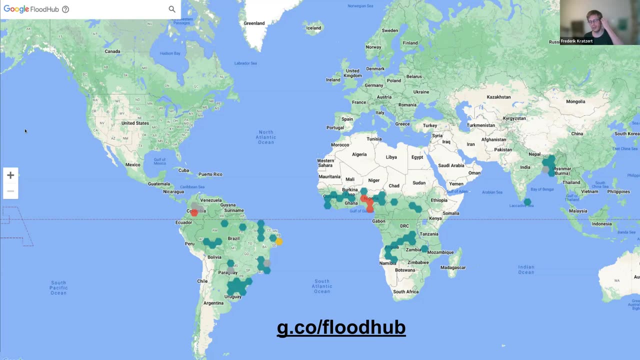 Yeah, so that's a bit frustrating as a reviewer in this field currently because you have to argue a lot And yeah, I hope it will change the future. With that, I'm at the end of my presentation. There's like one thing I want to mention here, which is that last week Google officially launched what we call the Flathub. 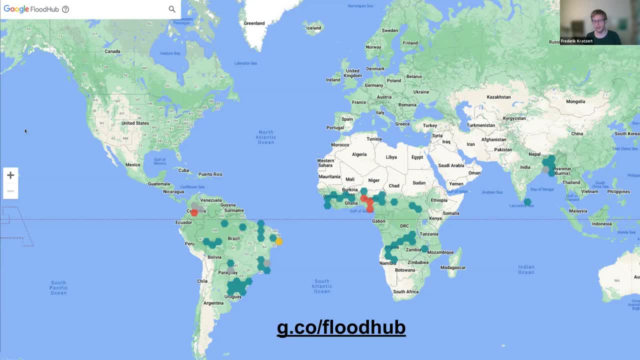 So this flood forecasting initiative that I'm working in. Previously we provided flood forecasts only in certain countries where we had like a contract with the government. These were mainly India, Bangladesh, and then also Colombia, Brazil and Sri Lanka, I think. 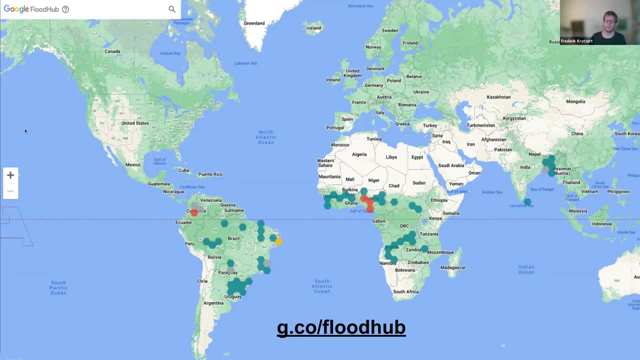 And these models were fed also with real-time observations of river water level and discharge And it was like not really scaling up to cover more countries because the contracts take a lot of time to get setting up the data pipelines with all of these countries. 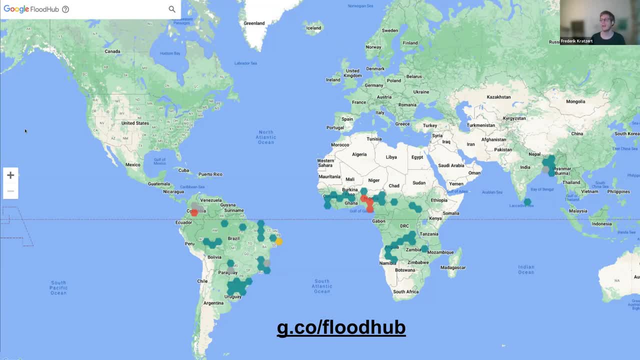 to get real-time measurements was not really working. So at Google we switched at basically training the models, as I described in this part in this presentation, as being only fed by meteorological observations that Katrin introduced, that we have globally available. 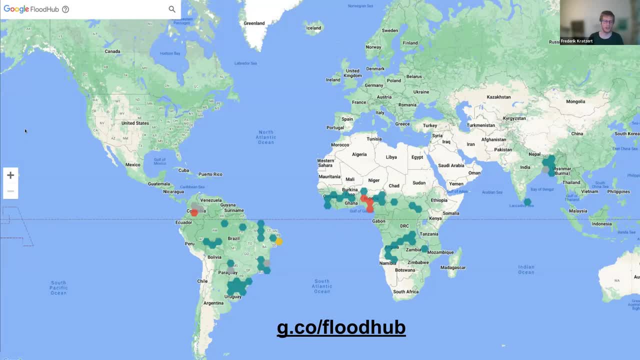 So we are now able, with this model, to actually give flood forecasts everywhere. right, The model is currently being rolled out and we will cover a lot of regions, a lot more regions than you see currently in the Flathub. 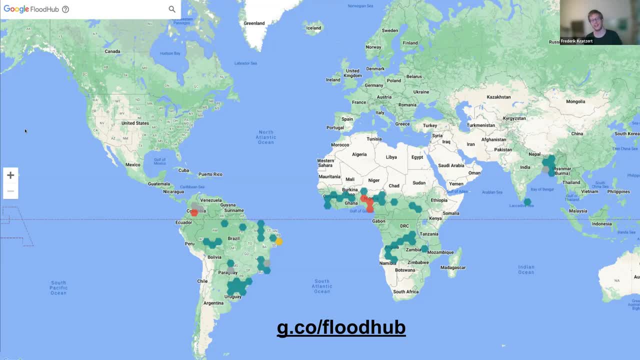 This is like our – it's not a beta launch, but it's – we released a couple of hundred pages just to see how everything works And then, gradually over the next months, we will cover more and more area. So this has been really exciting, because this is actually putting my research into operation. 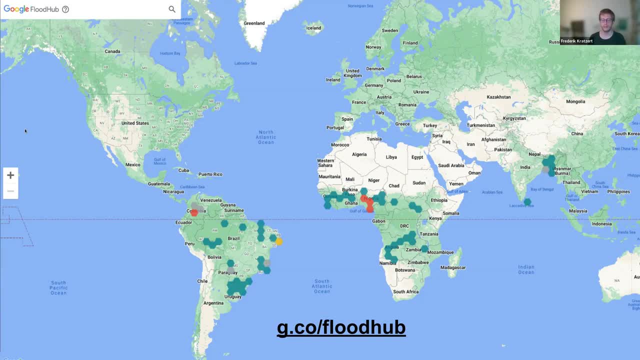 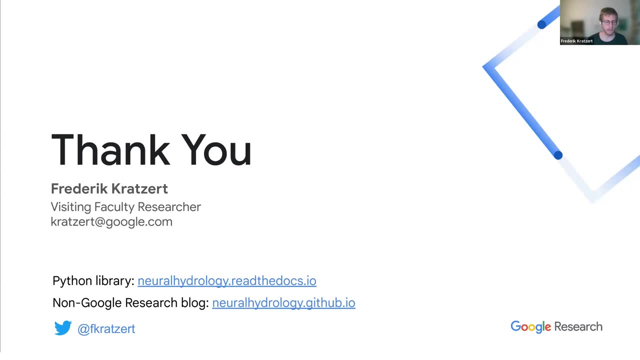 and it's now being accessible by everyone. And with that I'm at the end of my presentation. Great, Thank you. Do we have any questions? Perhaps I can start with a couple of questions. So you described the model and the LSTM. 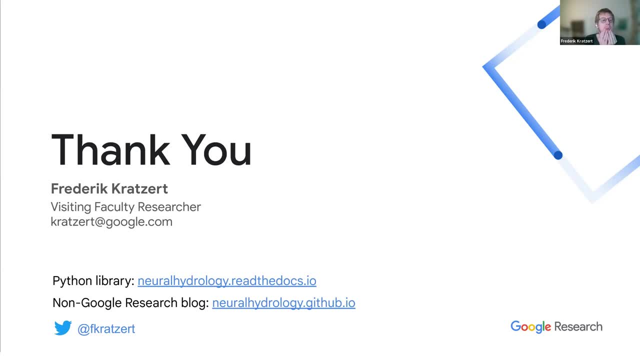 Perhaps you could mention a few more words on how the – what are the inputs, specifically the features, and how are they encoded? Right, Okay, So the –? we provide two different sets of inputs to the model. One are the dynamic time series, meteorological data. 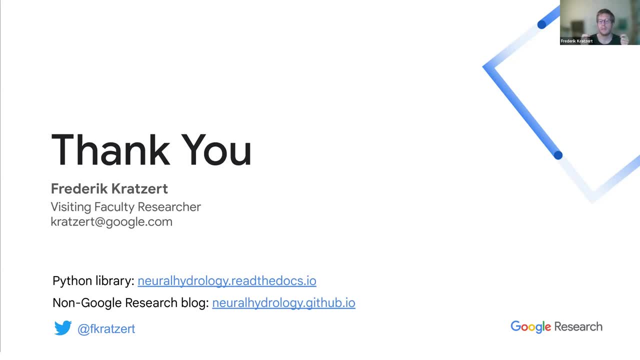 So this is, for example, the time series of precipitation over the last year, So actually it's one year. So to make the prediction for today, for the next seven days, what we do at Google is we provide the last year of meteorological data. 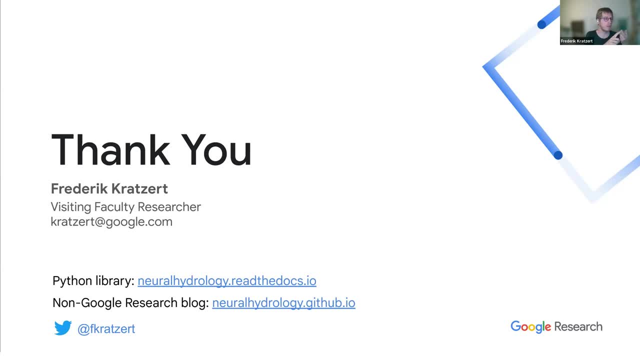 being precipitation, temperature being solar radiation, vapor pressure, a lot of the stuff that you get from these global climate models, of these global meteorological weather products. And the second set of inputs are what I call static attributes, but they don't have to be static actually. 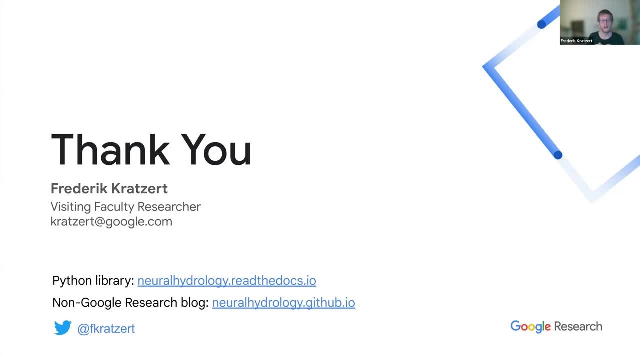 These are catchment descriptors. So this is the – all these features that are, the fraction of forest in the basin area, the soil properties, the area, the elevation, the slope of the terrain, So everything that we have – I don't know the amount of reservoirs in the catchment. 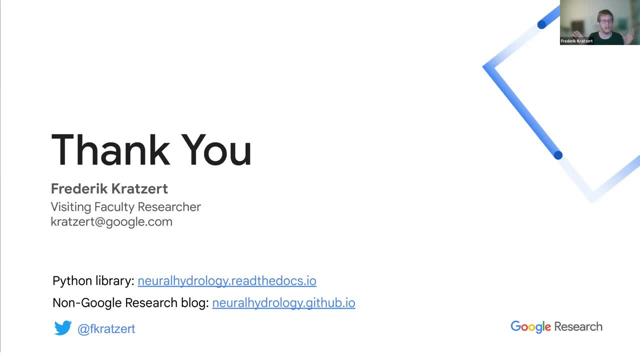 how many people live there, how many areas see it by settlements, all these kinds of stuff, everything that should influence the river discharge, that we can infer from some like globally available data sources. So we have these two different sets of features. 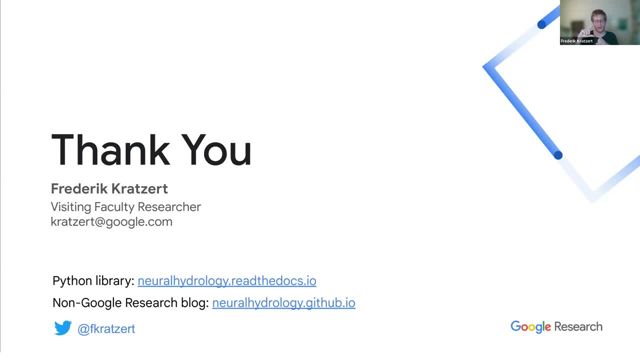 And I spent actually a lot of research time in how to best add static features to an LSTM, because LSTM are like sequential models- Sequential inputs- and static inputs are not sequential. It turns out that the best way how you can use static inputs 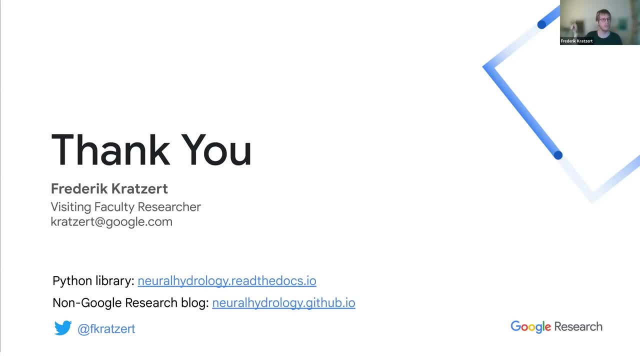 is to just concatenate them to the dynamic inputs at every time step And we actually – so we have an embedding network because we have like a couple of hundred static features, So we embed them to like a lower dimension. 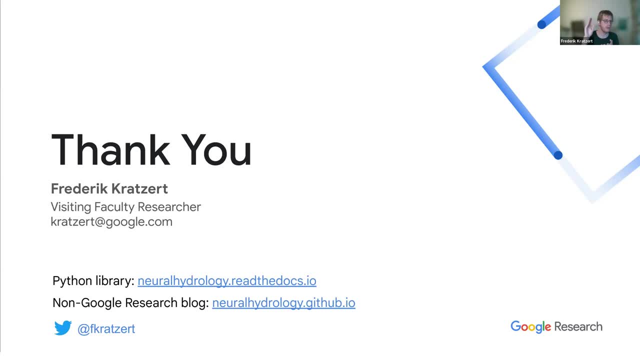 and then concatenate them to the dynamic features. but the dynamic features are not embedded at all. So it's the raw time series, like normalized, but the time series of metrological input data and embedded signal of the static catchment attributes. 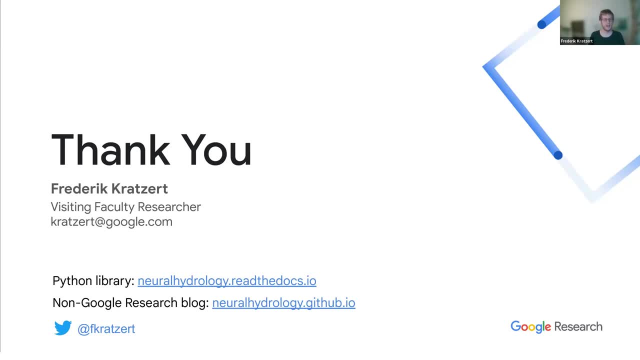 And that's it. We can – like the architecture is a bit more – like some more tricks. We can go into details if you want. You can see if there are other questions. What is the time resolution in the model? Yeah, so currently the time resolution in the model. 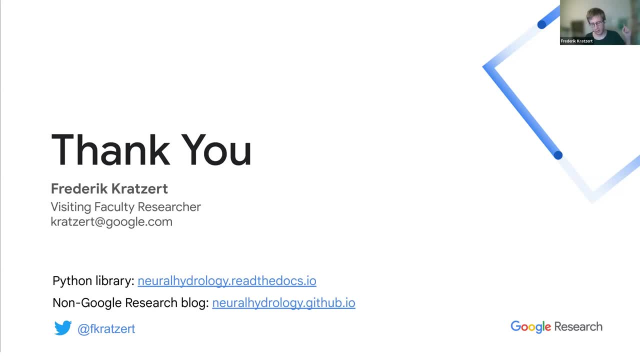 is of our operational model. The global model is daily. We have some local models that run an hourly time resolution And with hourly resolution, like providing one year of metrological forcing data, is like a sequence of 8,600-something time steps. 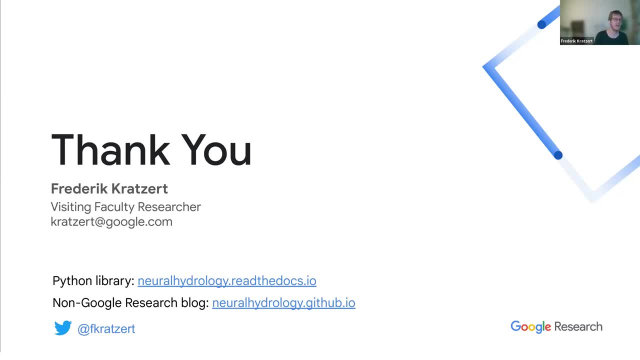 which is like not really what LSTMs like. It makes training harder. It gets quite a lot slower. So there's a publication from a colleague of mine. Basically, what we do is, let's say we want to do like issue and forecast now. 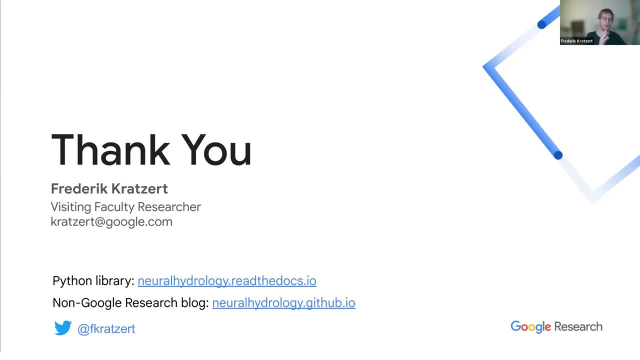 What we do is we summarize the past up to like, let's say, two weeks ago, using daily metrological data, And then, starting from two weeks ago, we only then we use hourly data because it shouldn't matter like at which hour of the day. 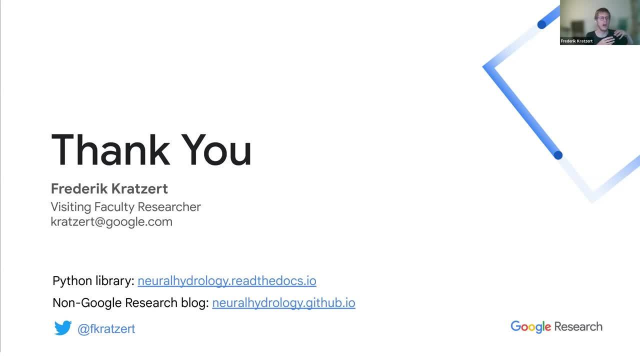 snow fell like six months ago, to know how much water there is now in the system. So we have basically like two LSTMs that are connected with like a state handoff. So we use the last hidden and set state from the first one. that codes the history of daily temporal resolution And then we have like a state transfer network that basically outputs the initial states of the hourly model And then the hourly model runs from just two weeks ago until now on hourly resolution And then also the forecast can be hourly. 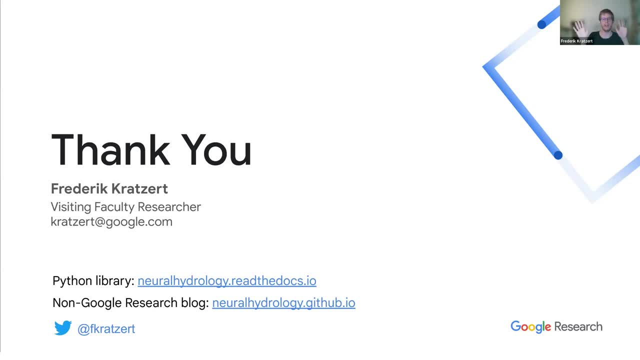 We do the same trick with like having two LSTMs, with like a state transfer for actually hindcast and forecast. So we have different sets of input available for forecast and for hindcast. So hindcast in hydrology or metrology is everything up to now. 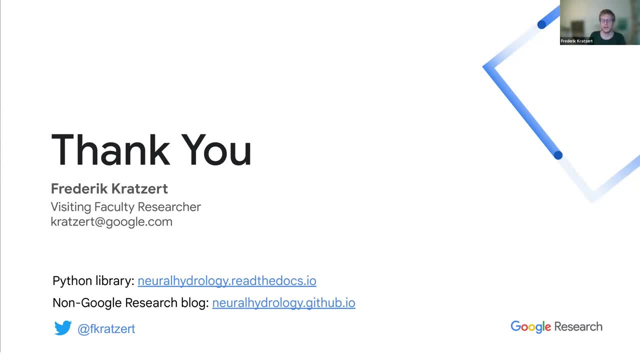 Forecast is like the future, So we have multiple sources of precipitation data and temperature data and whatever from like the past, But there are actually not so many different metrological, globally available weather forecasts, So we have different sets. 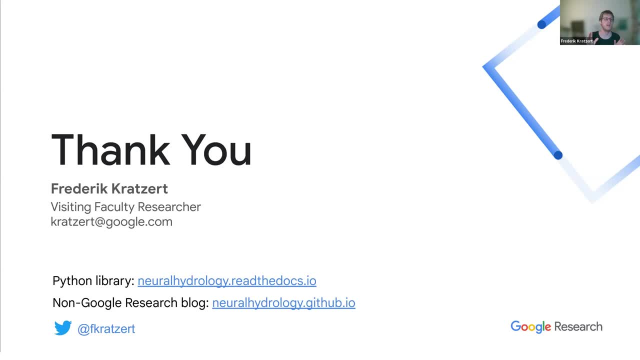 And they also come from different distributions, from different weather models. So we have two sets of input. So what we actually do is we have one LSTM that summarizes all the inputs up to now, And then we have a state handoff to what we call a forecast LSTM. 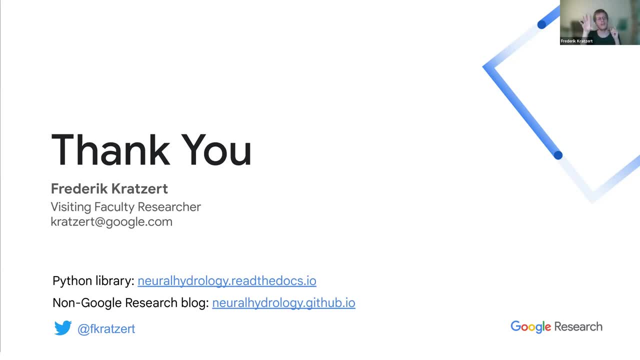 which is just another LSTM with different weights. that gets the forecast inputs and every time step outputs to this charge of this time step, this state And yeah, Okay. So we have a couple questions in the chat. Yeah, amazing. Would you like to read them aloud? 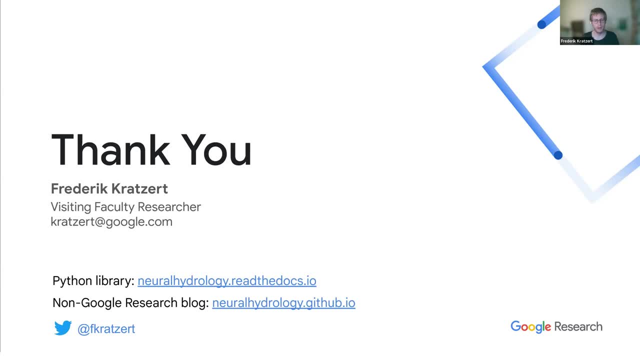 Or sort of summarize them. Yeah, I can start with the first And then maybe you already think about the summary of the next questions. So the first is by Scott, Wondering if you could explain a bit on the use of static attributes. 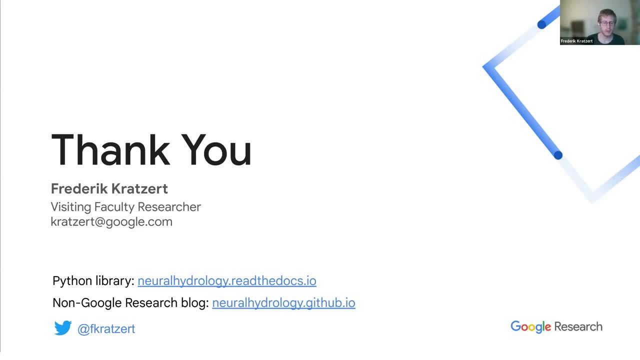 to learn across watershed types? Is there a certain way to use those that have proved most promising, And do they accommodate static attributes changing over time if multiple time periods are available? So yeah, Okay, Starting with the last part first. So, actually, what I said before, 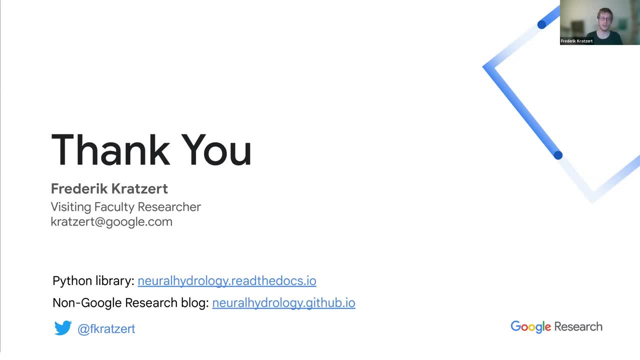 the static attributes don't have to be static. They could be, for example, a rolling mean being recalculated every week. So I said some of the static attributes will probably not change, like elevation, the slope or whatever, But we have some static attributes. 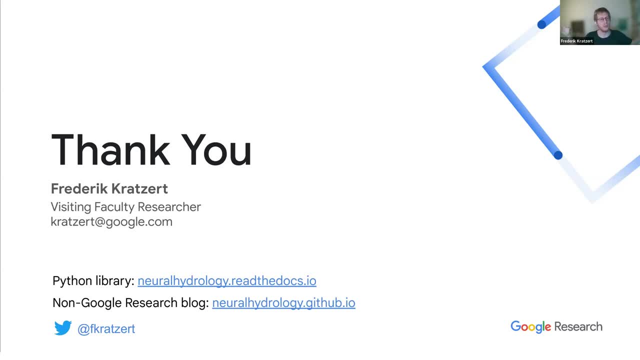 that are long-term climate indices, like the mean temperature over multiple years or days and the mean amount of precipitation falling in the region, because all of them cross-correlate with the vegetation and the environment in this area, So for sure you could recompute them. 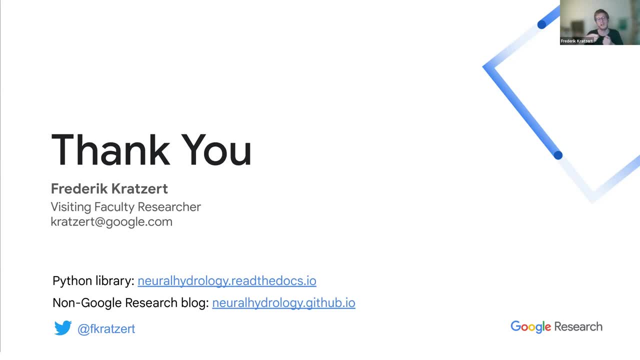 every three or four years or whatever, or like as a rolling window, and use this as static attributes, And we actually found this. The thing is that the academic data set that we use for most of our publications. there's no statistically significant trend in the data. 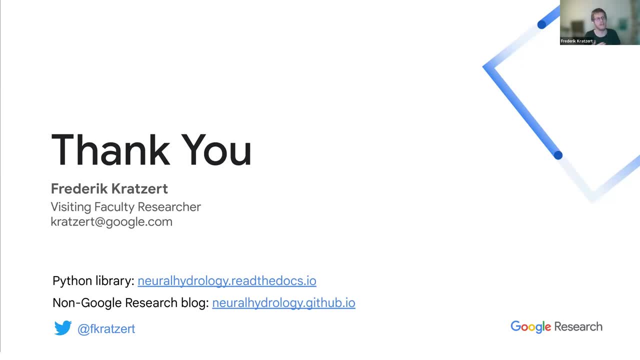 So there is no severe dryness happening or something that's actually changing. So actually for this data set, it was never useful to do this. I'm quite sure that if we would have longer data sets with a longer look back, 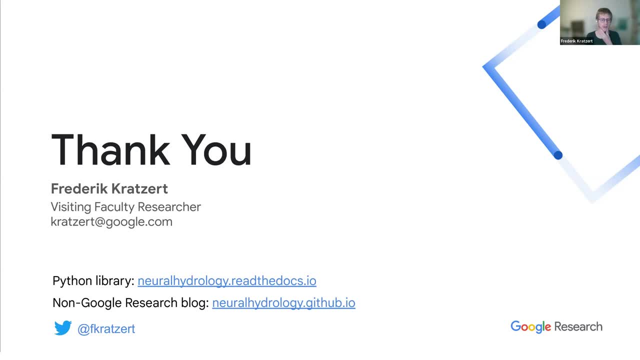 or also going into the future. that's definitely the right thing to do, Great. So perhaps I can summarize the next question. It's about Typical reviewer questions are: what can we learn with LSTMs? But rather, could you shed some light? 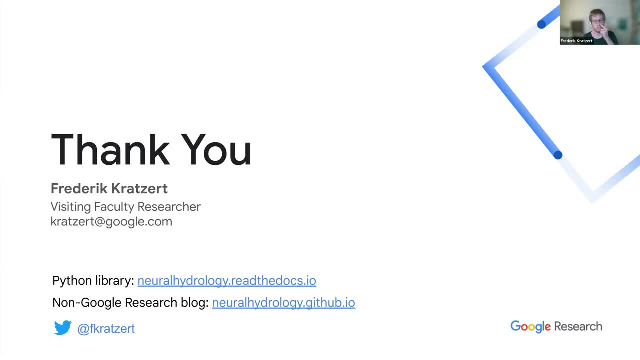 on what we cannot learn with LSTMs. Do you have some experience on that? Yeah, So we certainly cannot learn anything that's not available in the data right. So I don't know When we made this PAP experiment. 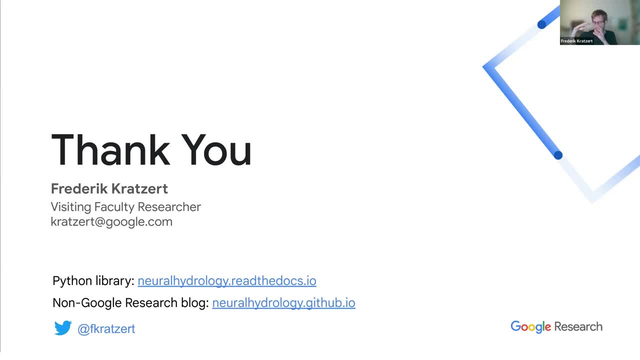 like this cross-border cross-validation on leaving out a set of basins, training on the rest. reviewers suggested to hold out certain climate zones. So training on all data but the high mountain basins and then testing the model how well it does in high mountain basins. 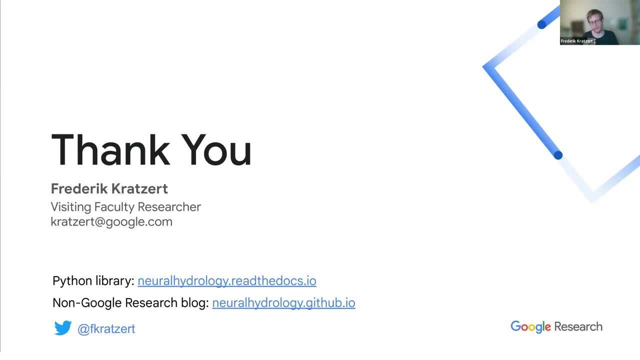 Certainly the model will not be able to do this because, to the extreme, if a model with an LSTM has never seen snow, it will not be able to model snow in any catchment afterwards. So what it can't learn is definitely anything that's not in the training data. 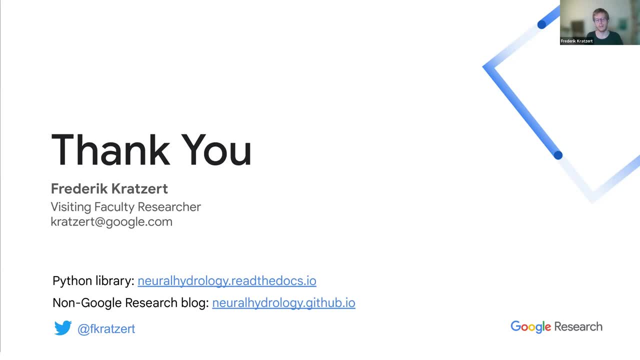 And I would say from the standard hydrological processes and the typical catchments. actually we have everything available if we look at the global context. So this data set that we train on at Google is like around 10,000 cages, I would say we cover basically any kind of natural environment. 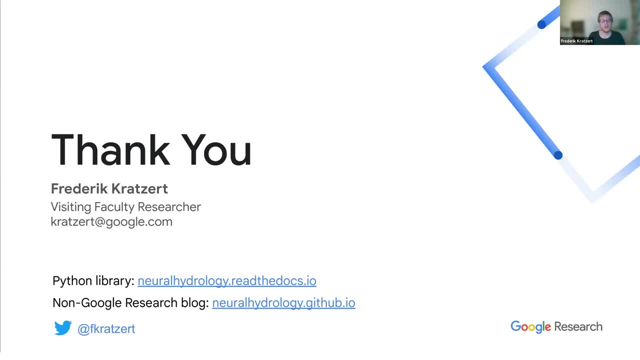 What it can't do if there's like a certain change in the catchment, for example, humans start to build like a huge reservoir and you have no way to inform the model that there's now an artificial reservoir in the catchment and that humans start to control the water. 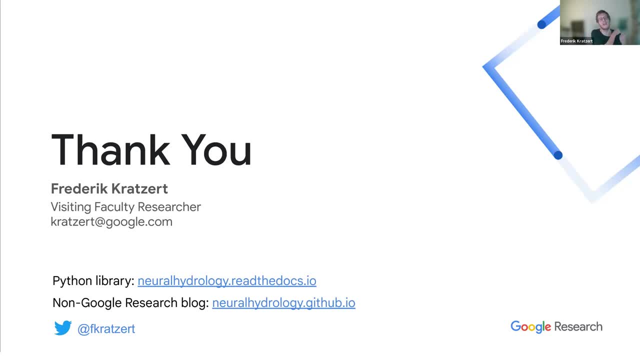 that is charged in the river and it's not the natural river or the river that, as it has happened in training, the model will not be able to account for that, But you could build the model in the first place, for example with like dynamically updating catchment attributes or whatever. 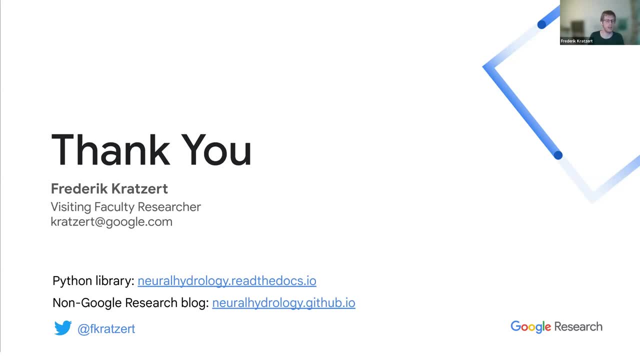 to inform it that a change in the catchment has happened. So yeah, On the case of like predicting discharge with the meteorological data, I'm not so sure yet that I know what this model is not able to do Like. it certainly has problems. 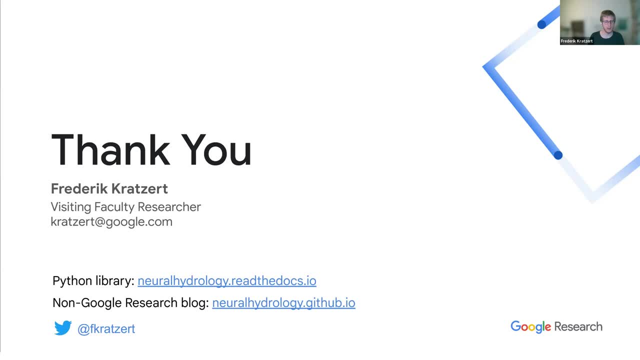 It is not really good in predicting inerrant catchments. So these spikes, high key catchments that are zero most of the time then have individual spikes. But these are also very problematic for any other kind of model, also for classical hydrology models. 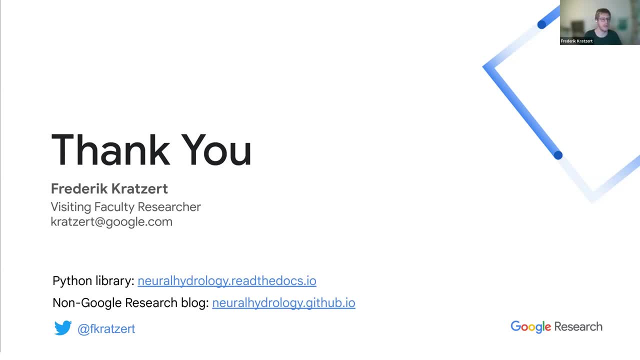 And also there the LSTM is better than hydrology models, but I'm not happy with the performance of the model there, So there's certainly work to be done. Next question is about GRUs. Did you compare GRU with the LSTM? 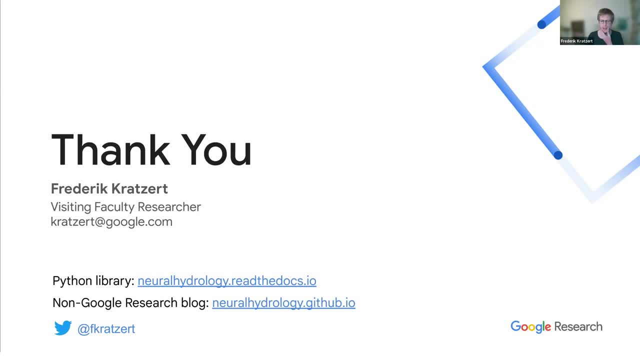 Yeah, we did. There are also some publications of other groups. So in general, the GRU is: yeah, it performs worse. It's not like a huge difference. The problem that I have with the architecture is that, if you know how the architecture works, 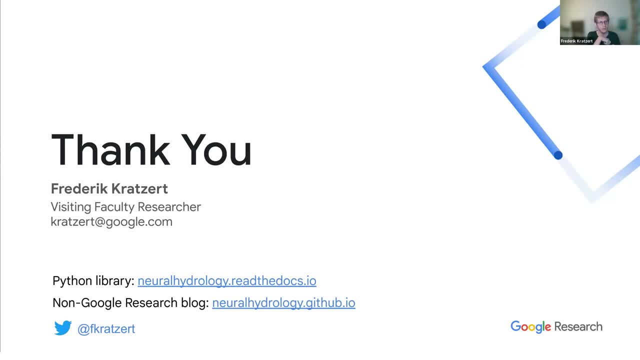 you can only add something to a sales state if you remove the old content of the sales state. So you're not as easily able to accumulate the signal in one cell. But this is exactly what we want to do. So if we want to accumulate snow, 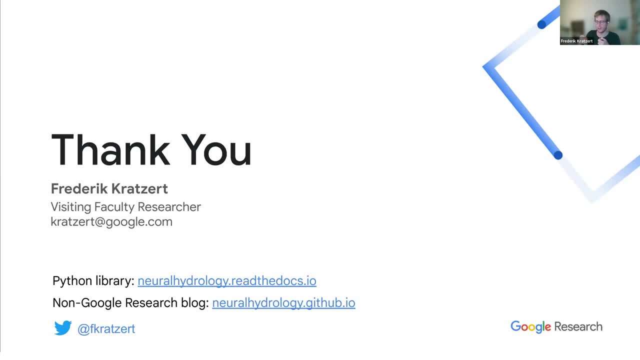 this is like adding the precipitation input at every time step where temperature is below zero, for example. So with an LSTM that can be modeled with a single cell, With the GRU model, you need at least two cells and then always write the content of this one cell. 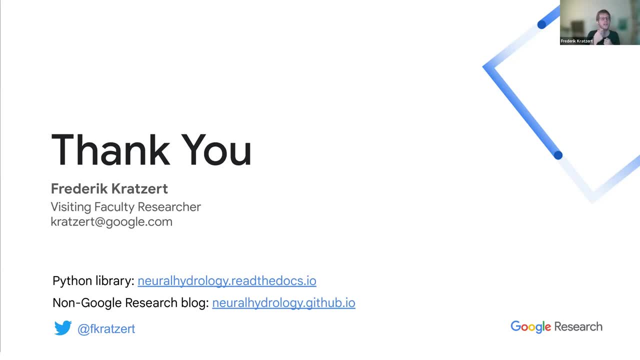 in a different cell and add something, And then, because to add something to a GRU cell you first have to add something, You first need to remove something. Performance-wise there's very little difference, But because of this we stick with the LSTM. 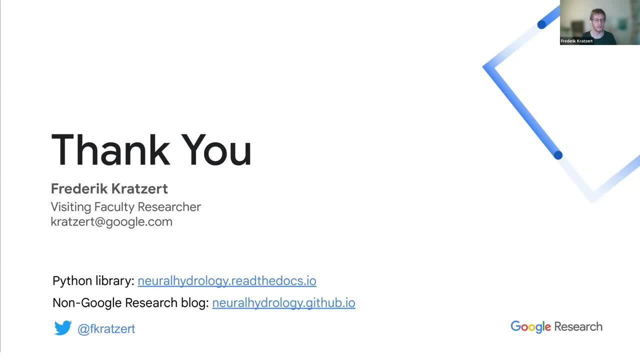 because I like the fact that you don't need to shuffle around information so much. I have a follow-up question on that: Did you compare with any other model architectures? You can model sequences with a transformer as well, and also with a common, So actually yes. 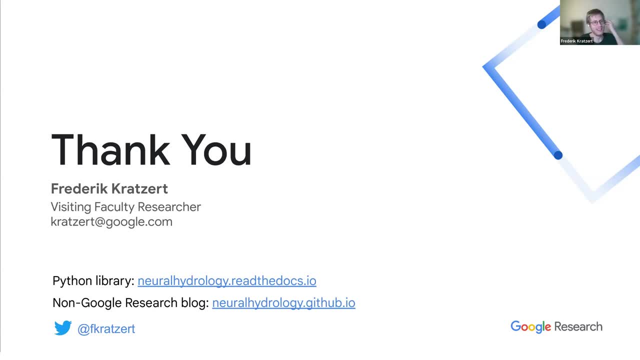 The transformer question. I thought it would come up here. Actually, we did it a while ago and we didn't repeat this experiment with our most up-to-date, largest data set, So it's certainly something that is on the to-do list. 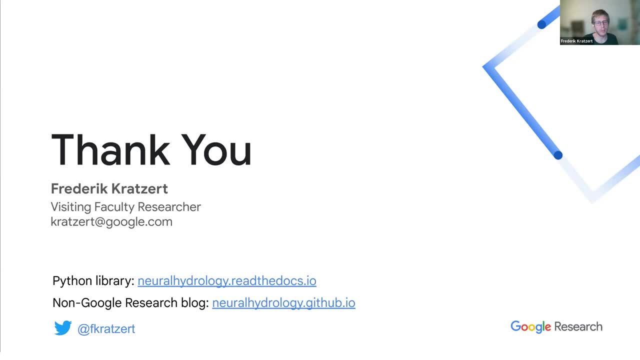 On this academic data set that we used to do all of our paper tools. transformers were considered like they were better than hydrology models but significantly worse than LSTMs Being in the order that it's not like a huge gap, as with the hydrology models. 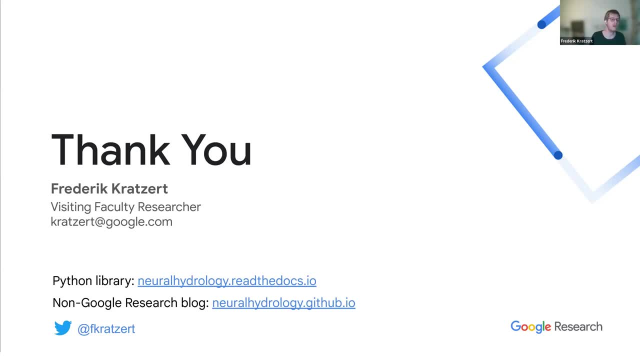 but it was consistent and significant. So maybe it's because the data was not too much and the inductive bias of the LSTM model for this application was still the dominant factor. But this is definitely an experiment that we are about to repeat, Because I don't know. 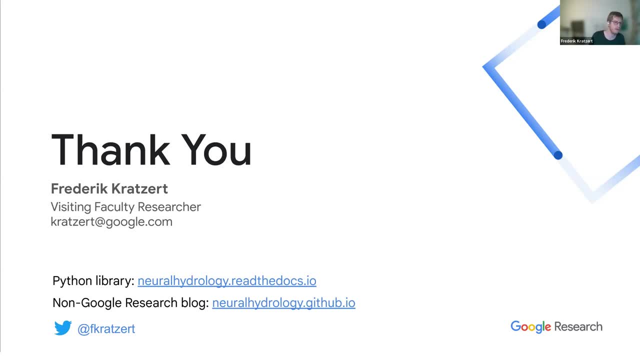 from all other fields. at some point there should be, Yeah, convolution networks. we also tried them. They were not particularly good for temporal convolution. Okay, the next question is: do you have some insights about why LSTMs perform poorly? 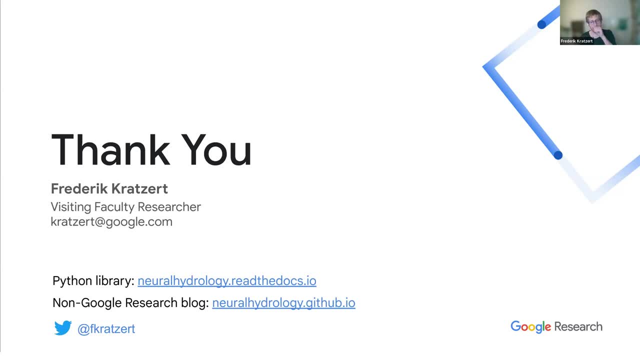 in specific basins or regions. So yeah, one is the arid basin stuff. This also is coupling to the next question, which is why she learning models are failing in arid areas. Again, also hydrology models fail there. So it's like the kind of basin. 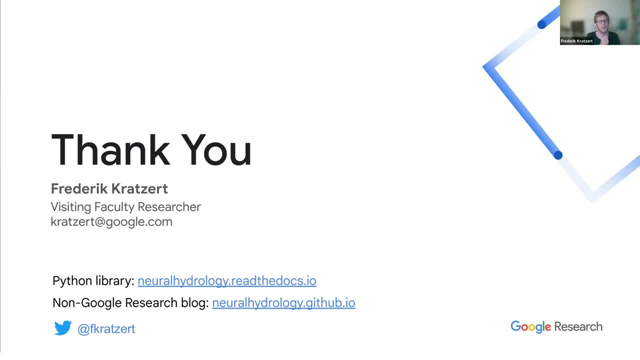 is particularly difficult, I think so let's just need some explanation. So the time series is zero most of the time and then has, like, individual spikes. The NSE is a metric comparing the simulation to the mean prediction. The mean prediction here would be like: 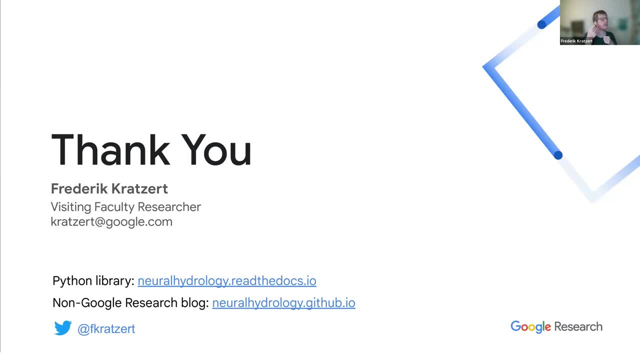 to the baseline model, the R-square. the baseline model is the mean prediction. So the mean prediction would be close to zero. so this is very hard to beat. if you're predicting arid basin that it's like 364 days a year zero. 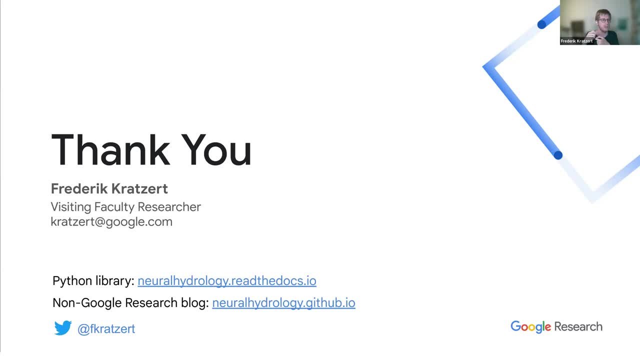 You get very easy of that metric just by being slightly off, because just predicting zero is already. it provides a very good metric right. And then what happens here is that you get all the time like little precipitation, some temperature, and then at some point 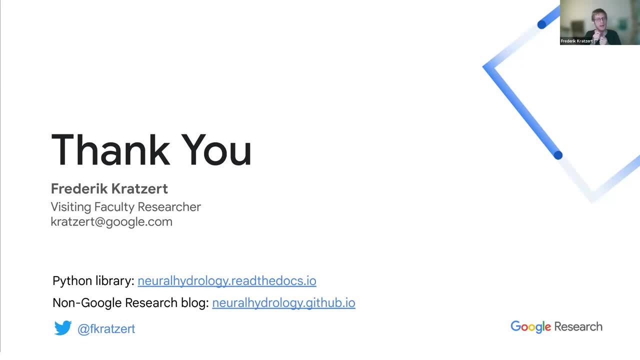 there's an immediate spike. There's an immediate spike right, And actually hitting the spike is kind of easy for the model, but getting the right magnitude of the spike is what's the problem, And here I would also hedge the results a bit. 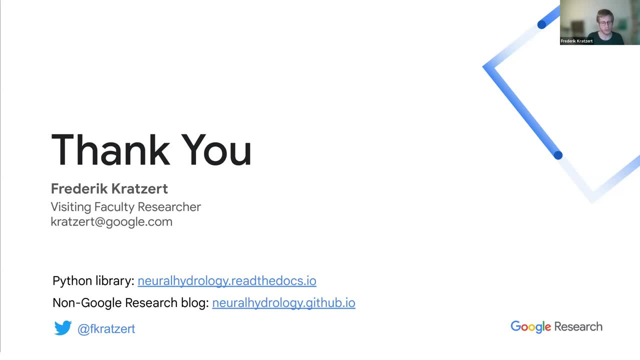 because the ground truth data that we have to observe discharge- this is a very understated measure, right, The value that we have there in the data set doesn't mean that this value is the truth, because measuring discharge specifically during floods is very challenging and there's like 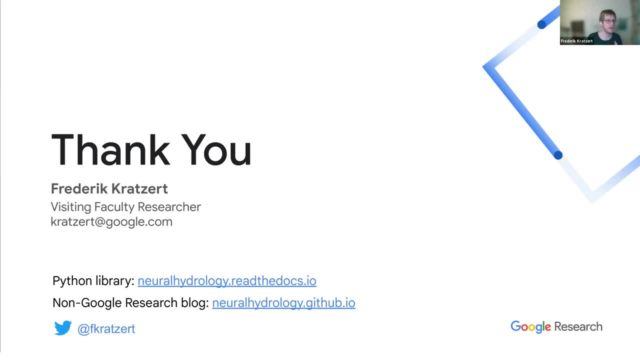 I think there are publications showing that we have at least a 50% error in peak discharge events. So yeah, it's a bit of a question like how good do we want to get, because at some point we can't get much better. 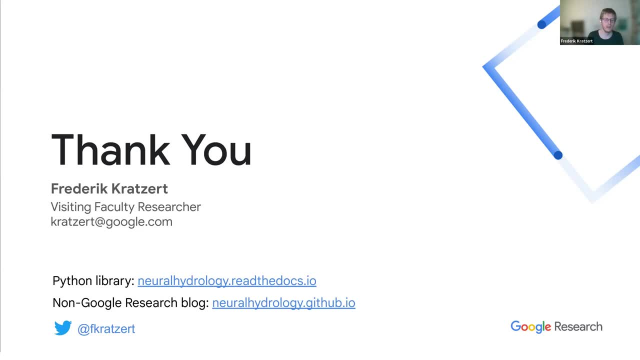 because it's just within the uncertainty of the data, But still there's like still, I would say, error base in general is the most problem And I think, okay, why? Maybe because the training signal you get is very little, because it's zero most of the time. 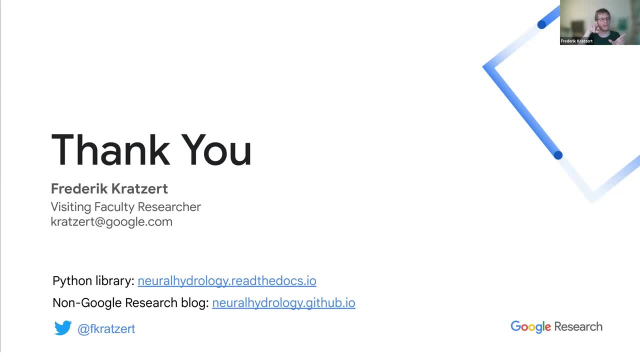 So all input sequences go to the same output value of zero and then you just have very few samples that have an actual value. that's different, And maybe also because it's just hard to learn the threshold of what needs to happen, that you now have to discharge. 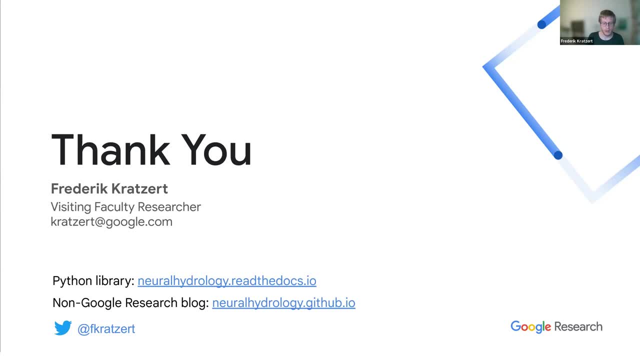 Yeah, And then specific regions and basins. So in general, I would say that the most problem that I see with all data that we have is about the quality of the data. Whenever we have high quality discharge data, we get usually very good models. 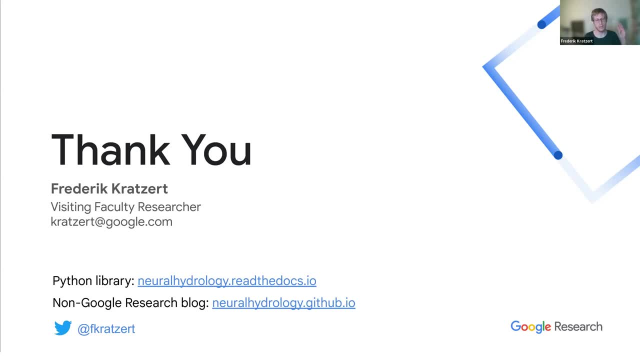 So I would say, if we have a region that is considerably bad, it's most of the time because the data is bad. Yeah, So perhaps we should round off the seminar there. Thank you very much for this presentation and for this discussion session. 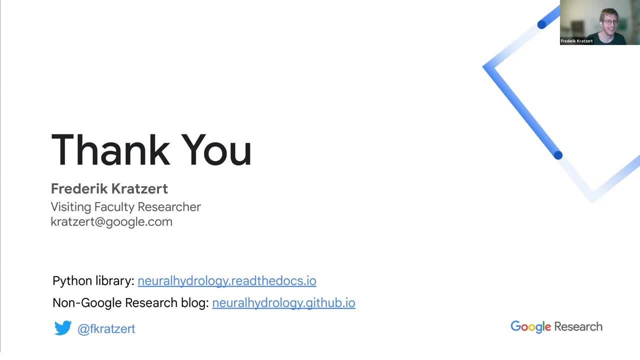 which was performed mostly in the chat, But I think it works. So, for those of you who wants to know more about Google's work, I know there's an interview with Stellan Nebo, who perhaps is a colleague of yours. He's actually my manager's manager. 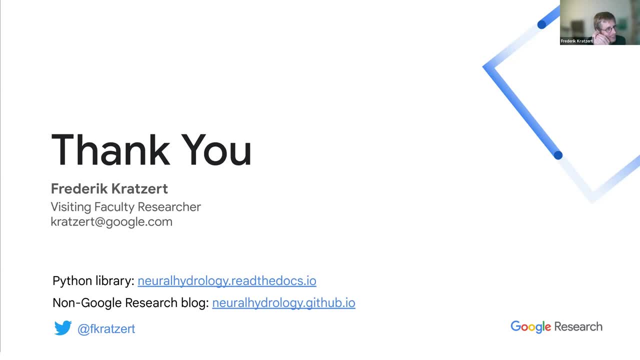 Yeah, yeah, He's my boss. Yeah, So there's an interview with him on the Talking Machines podcast from a while back. So I guess, if you want the updated information, you should have attended this seminar instead. Otherwise, welcome back in one week. 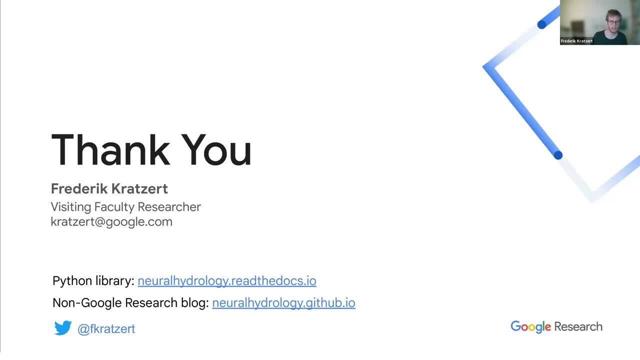 We'll have Mohammad Osama, who is at Aptiv, who will be presenting next week. The topic next week will be robust risk minimization for statistical learning from corrupted data. So welcome back then, And thank you very much for this interesting talk. 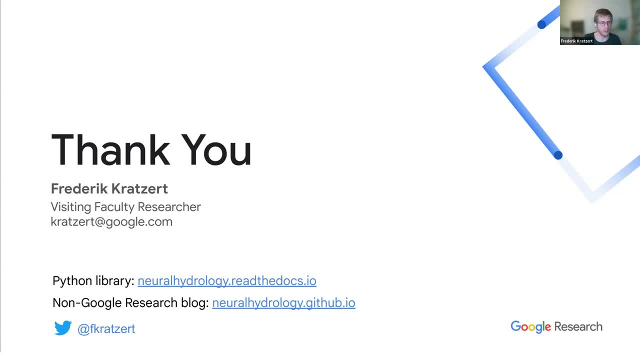 Yeah, Thanks again for inviting me. Just like one last thing: If there's any other question, feel free to contact me via email or Twitter. I'm happy to answer any question. Great, Thank you. Bye-bye everyone. Bye-bye. Bye-bye, Bye-bye, Bye-bye.